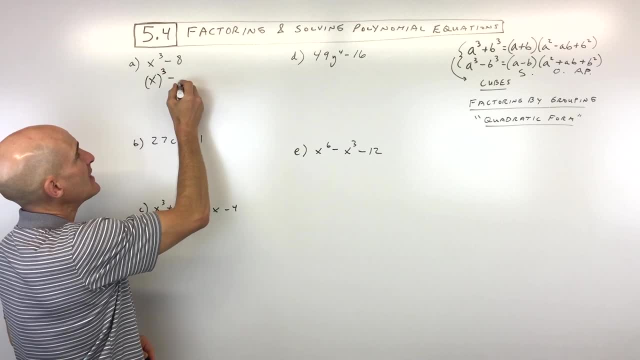 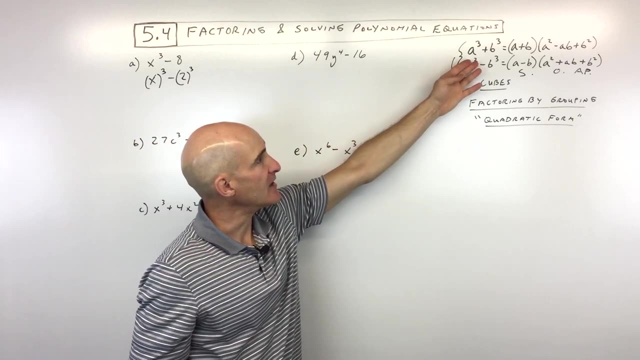 this is obviously a perfect cube. It's x times x times x. 8 is a perfect cube. It's 2 times 2 times 2.. So now what we can see is that our a value in this formula okay, is going to be x and our b. 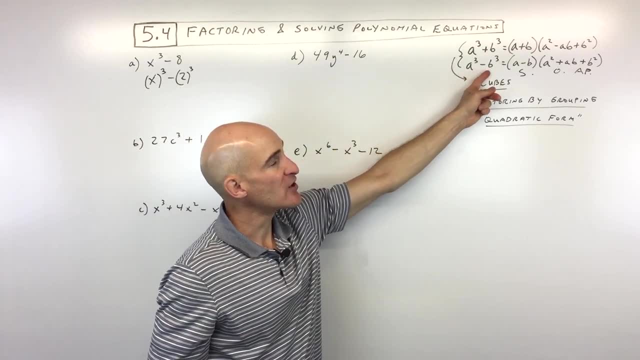 value is going to be 2.. We can see it's a difference of two cubes, so we're going to want to use this second one here, And then what we're going to do is we're just going to expand it. So it's going to expand to. 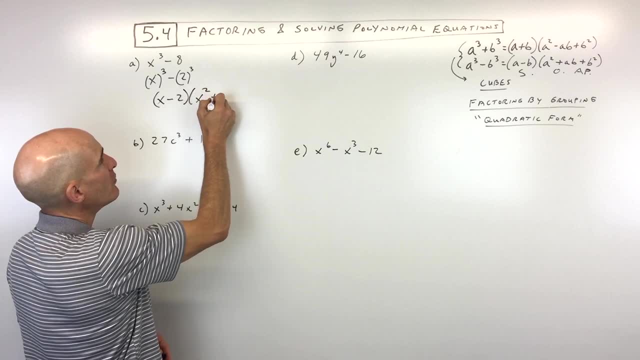 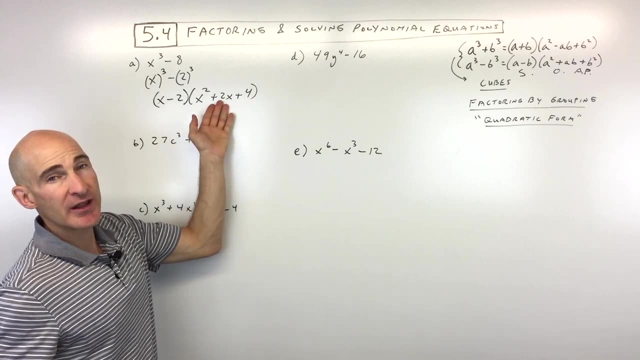 x minus 2, x squared plus 2x plus 2 squared, which is 2 times 2.. That's 4.. Now you're not going to be able to factor this trinomial here any further. That's as far as we can go, But remember the first. 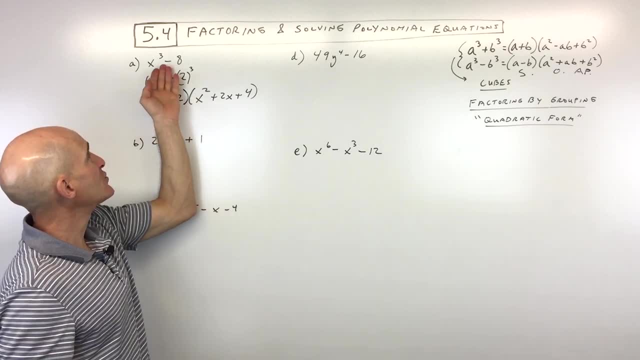 step is always to do the greatest common factor when you're factoring. But if you find that you have a difference of two cubes or a sum of two cubes, just take the q root of each of the two terms to identify your a and b values. So you're going to want to use this second one here. 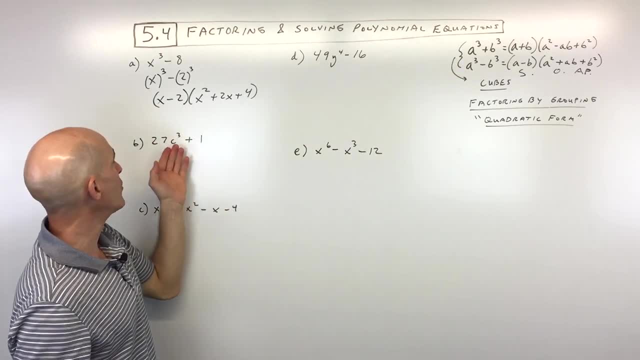 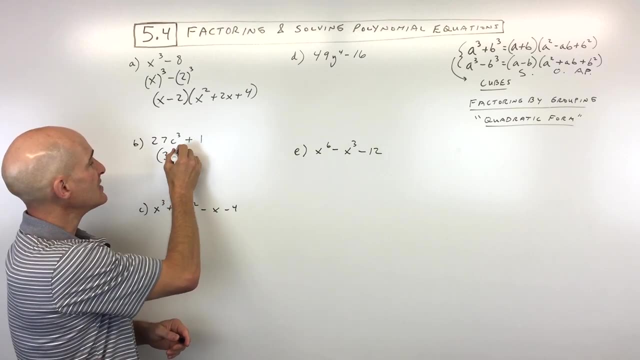 Let's do another example so you can see how that works. So let's look at letter b. So when you look at letter b here you can see that 27c cubed is really like 3c, the quantity cubed, So 3c times. 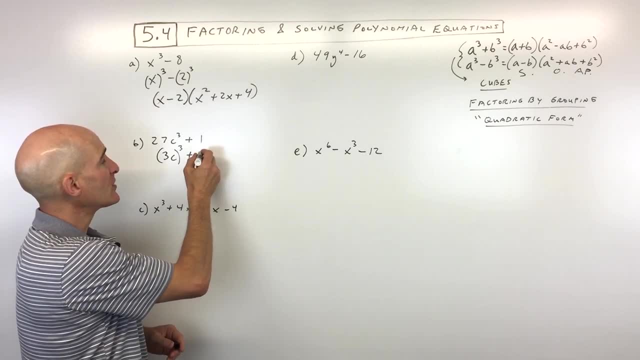 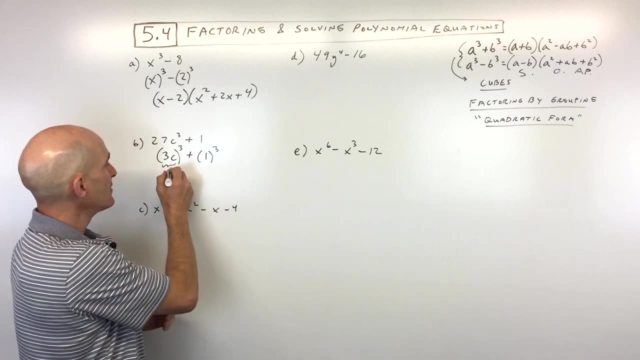 3c times 3c- 1 sometimes is often overlooked as a perfect cube, but 1 times 1 times 1 is going to be 1, right? So we can see our a value is 3c and our b value is 1.. So all we have to do now is 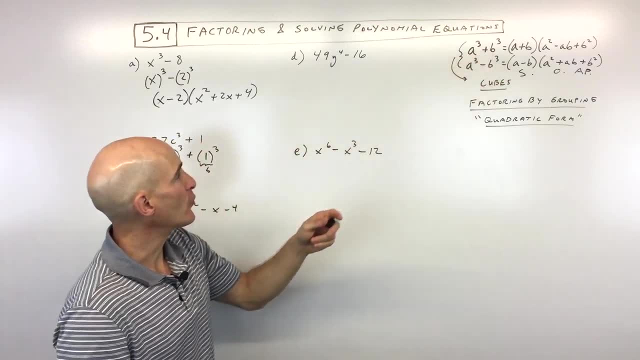 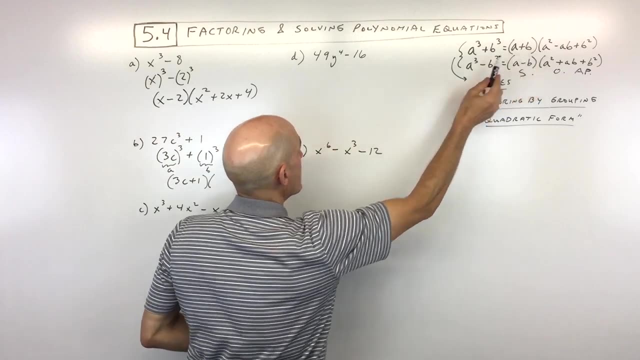 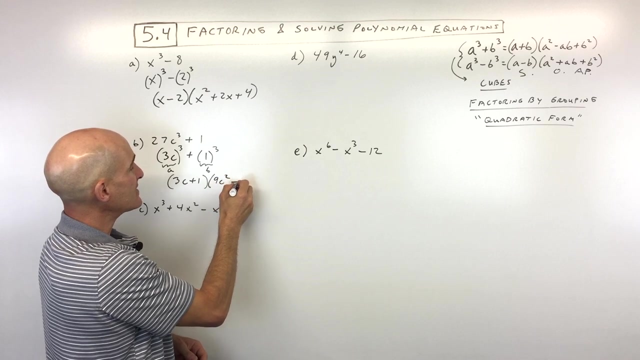 substitute into our sum of two cubes this top formula and that's going to come out to 3c plus 1.. So that's a plus b, a squared, which is 3c times 3c, so 3c times itself. so, squaring it, that's 9c squared minus. 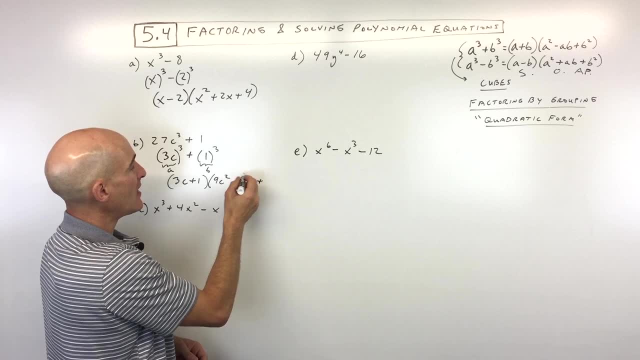 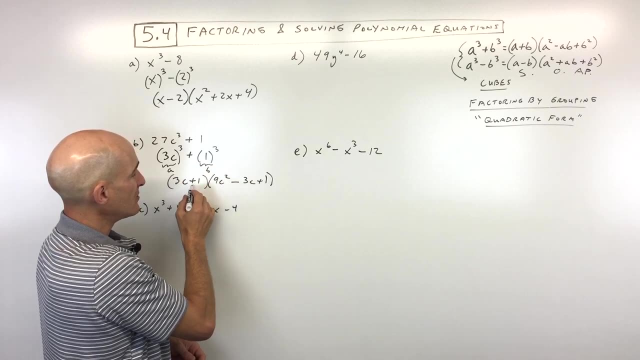 a times b, 3c times 1 is 3c, plus b. squared 1 times 1 is 1.. So you've got the same opposite, always positive. We're adding: so it's the same opposite sign, always positive, and you've got. 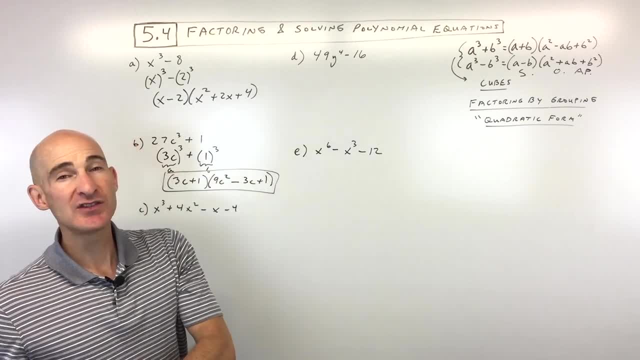 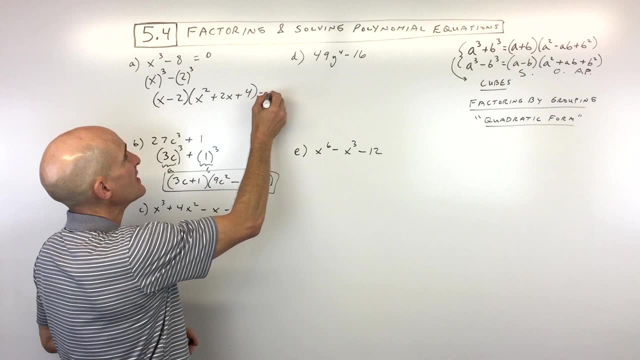 fully factored and that's it. Now, if you were solving these equations, if it said: you know, say, for example, this was equal to 0, what you would do after you factor it is, you would then take each factor, each group, and you would set it equal to 0 and solve, And that's how you would. 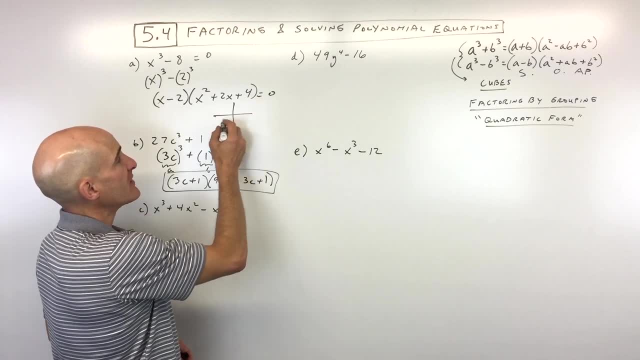 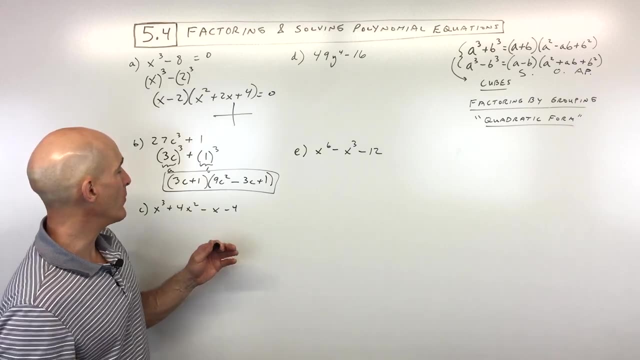 find your 0s which represent the x-intercepts where a polynomial is going to cross the x-axis. So we're going to use that later on in this chapter as we keep going through. but we're just reviewing factoring here, so you have those skills to find the 0s which are our. 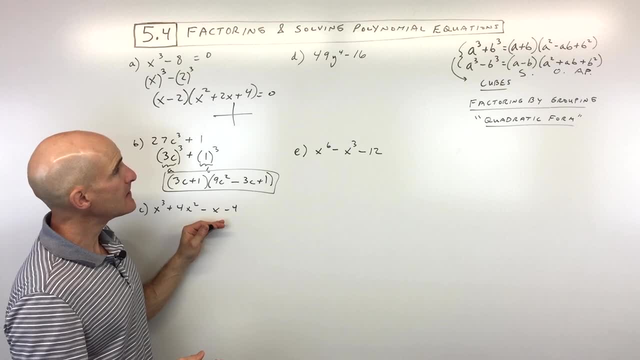 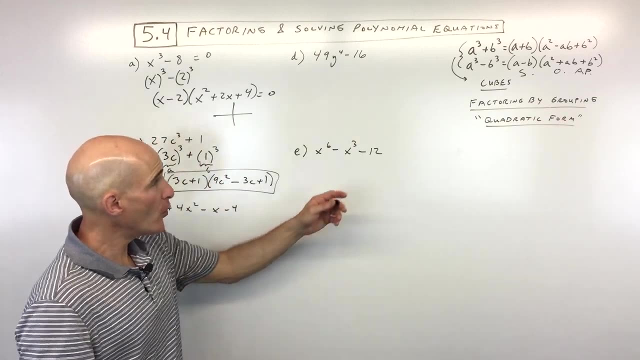 x-intercepts. Okay, now we're jumping down to letter c, and here what we're talking about is factoring by grouping. So most likely you did talk about this in Algebra 1, but you know when to use factoring by grouping: when you have four terms. okay, Four terms. Remember, the terms are separated. 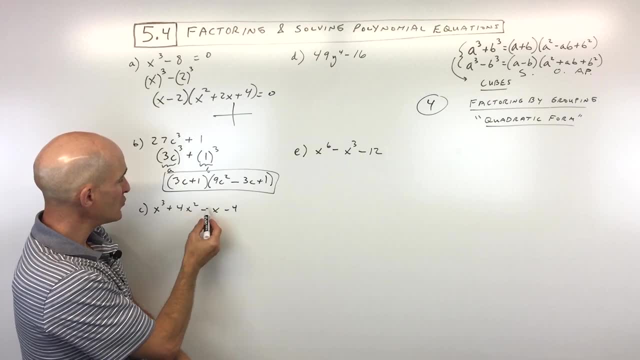 by plus or minus, so it's like four groups. So you can see, here we have one, two, three, four terms. What we're going to do is we're going to group the first two terms and we're going to group the last. 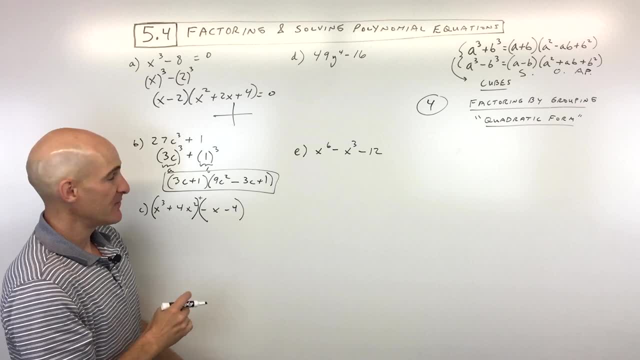 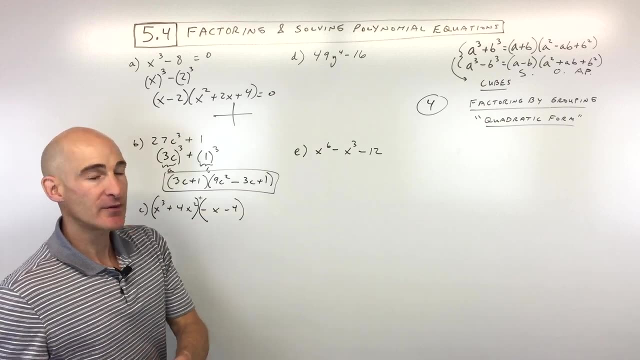 two terms, but there's really a plus sign in between here. okay, These are not multiplied together, They're just x cubed plus four, x squared plus negative, x minus four. I'm just grouping them into two groups. okay, Now what we do is we factor out the greatest common factor. So here you can see. 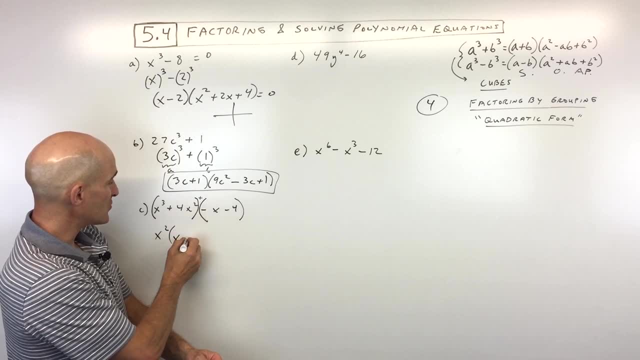 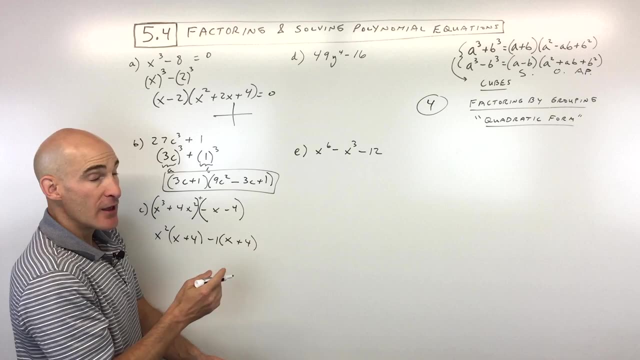 we can divide out an x squared out of both of these two terms. That's going to leave us with x plus four. Here we can factor out a negative one. So I'm just going to factor out a negative one. That's going to give us x plus four, If all goes well. notice what's in the parentheses. 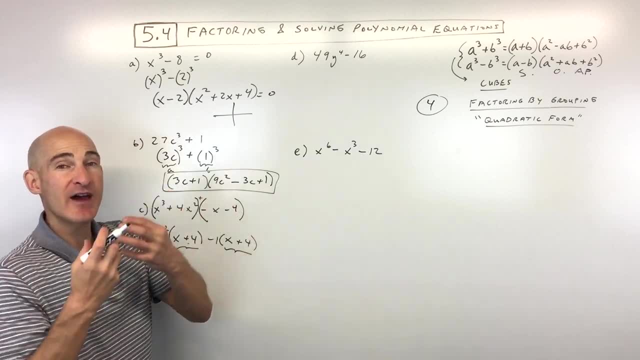 It's the exact same. See, it's x plus four. So what we can do is we can then factor out the x plus four as a greatest common factor. See, if you were to divide this whole group by x plus four, you'd be left with x squared. 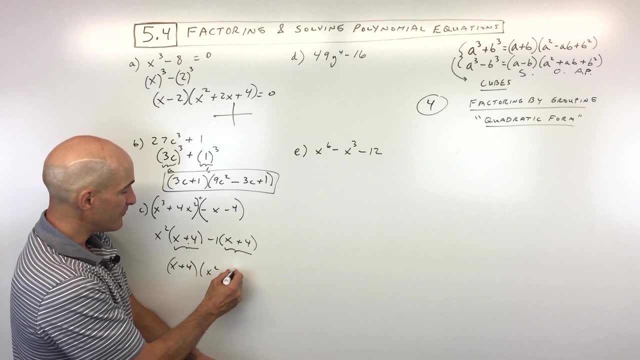 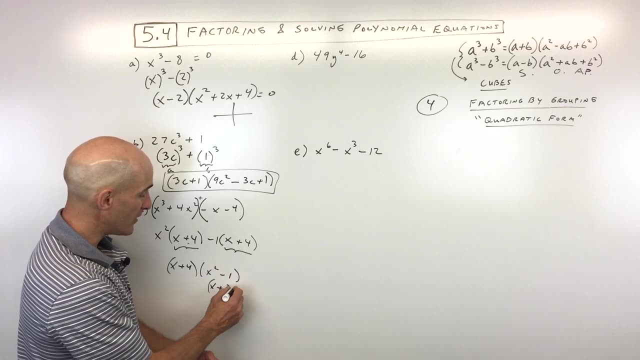 And if you divide this whole group by x plus four, you're going to be left with negative one. Now notice: this is a difference of two squares: x squared minus one. This is actually going to factor to x plus one and x minus one, and we'll just bring down our x plus four. So if you were 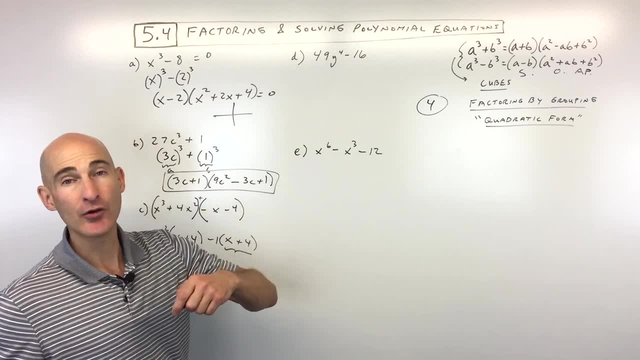 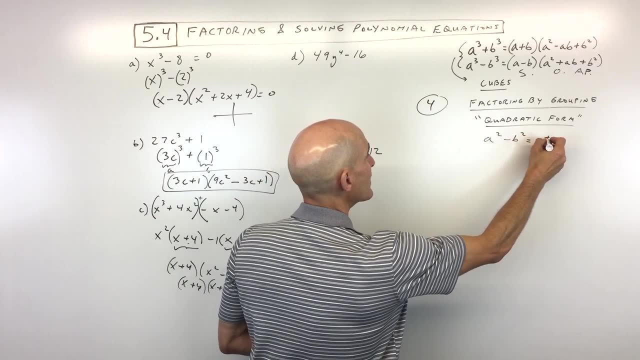 to multiply all this out, you'd get back the original polynomial. okay. Now remember, with the difference of two squares. just a reminder: this is a squared minus b squared. it factors to a plus b, a minus b. okay, So it's a sum and difference pattern. 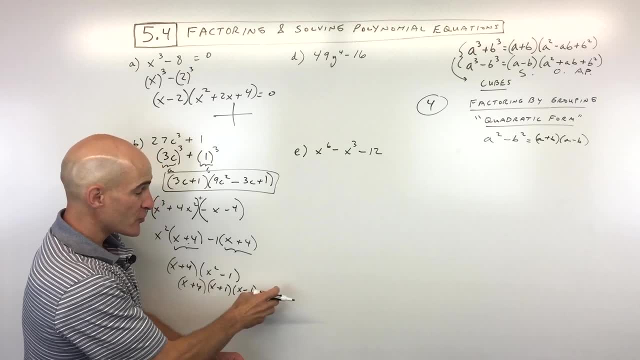 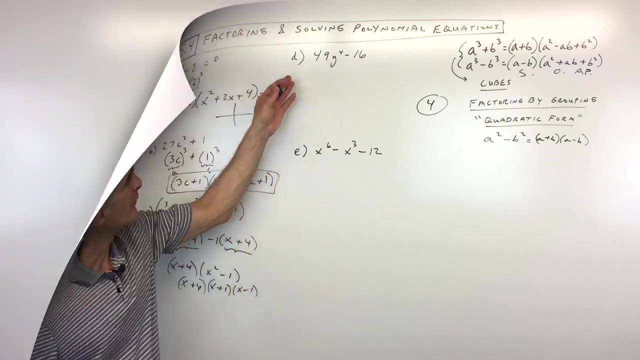 Now, if this was equal to zero, then you would set each factor, each group, equal to zero. make a mini equation, basically set those to zero, solve, and those are going to be your x-intercepts where it crosses the x-axis. Okay now if you want to learn Algebra 2,. 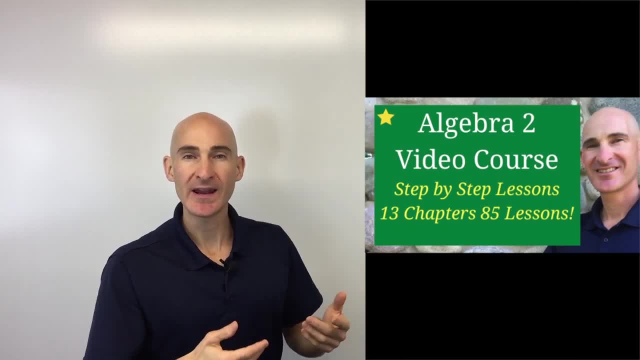 check out my Learn Algebra 2 video course for sale, where we go through 85 video lessons that take you step by step by step through Algebra 2. We go through the important formulas, steps, as well as numerous examples to help you master Algebra. 2. Click the interactive card or 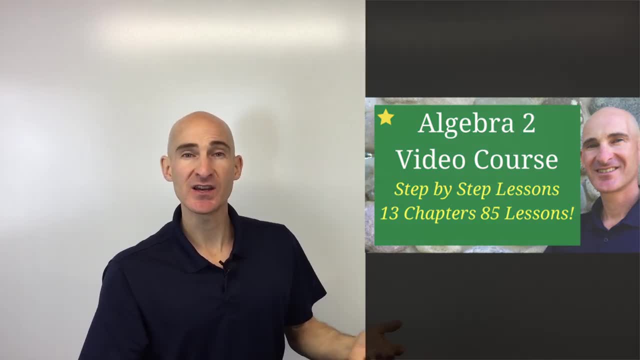 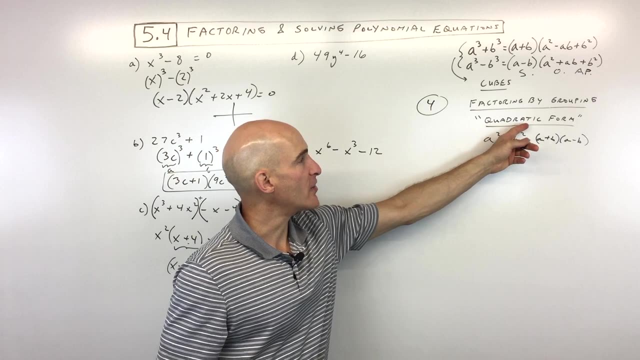 the link in the description below to go over and check out some of the free lessons. Otherwise, let's get back into this current lesson. Okay, now for letter d and e. what we're talking about is the quadratic form, So this is like recognizing how to factor these when they're in the quote. 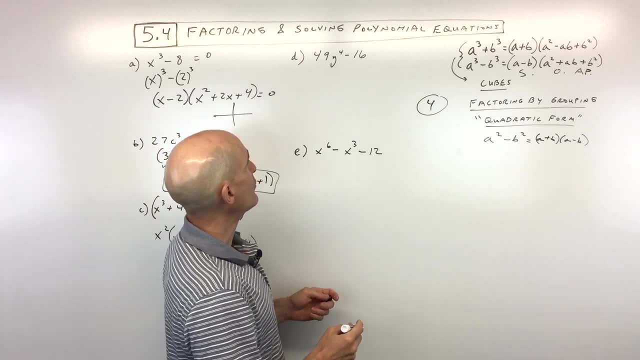 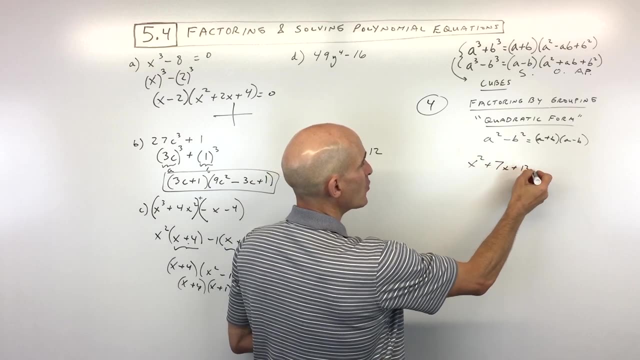 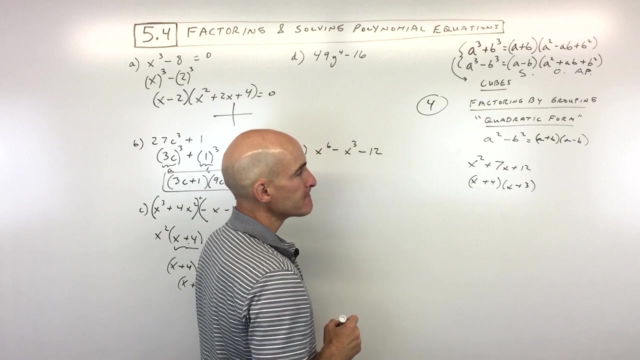 unquote quadratic form, and I'll just give you a simple example here. Say, for example, you had something like this: x squared plus 7x plus 20.. We know how to factor this. This is just going to be x plus 4 times x plus 3, right, But what? 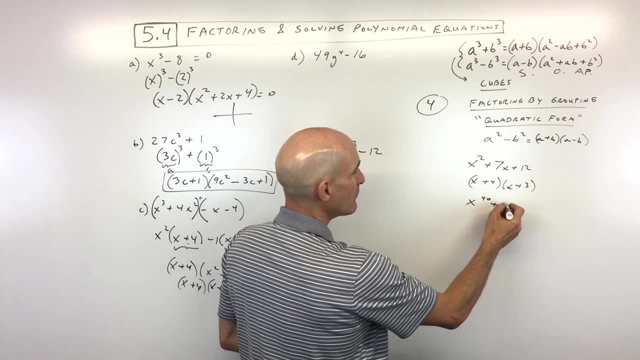 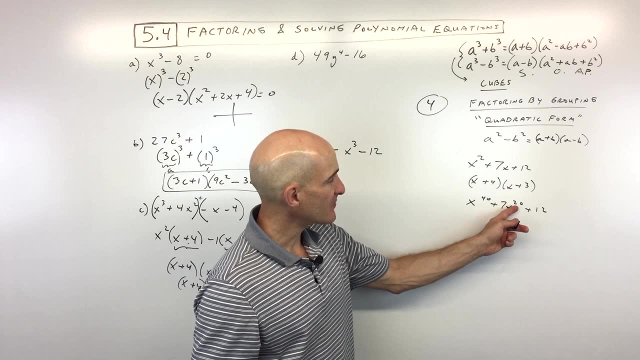 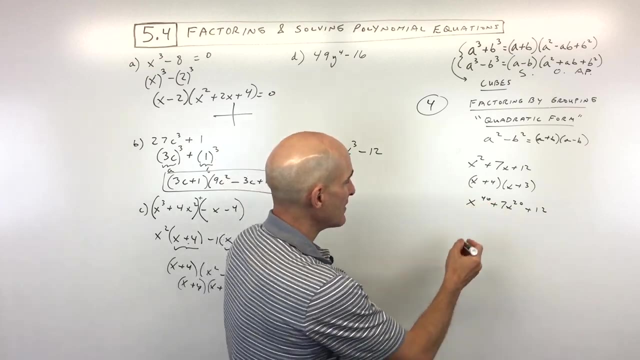 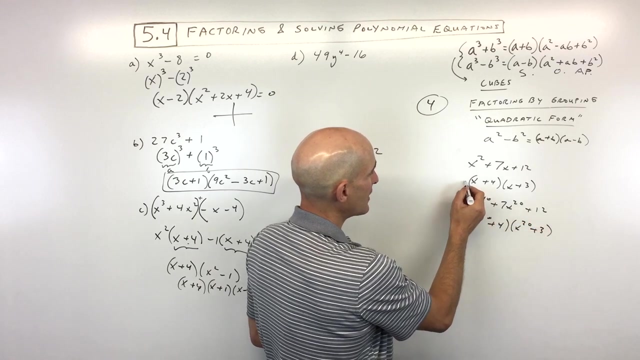 happens if this was x to the 40th plus 7x to the 20th plus 12?. Now what makes this in a quadratic form is you see how this middle exponent is half of this leading exponent. This is going to factor x to the 20th plus 3, just like if we were factoring this one up here. See how it was like. 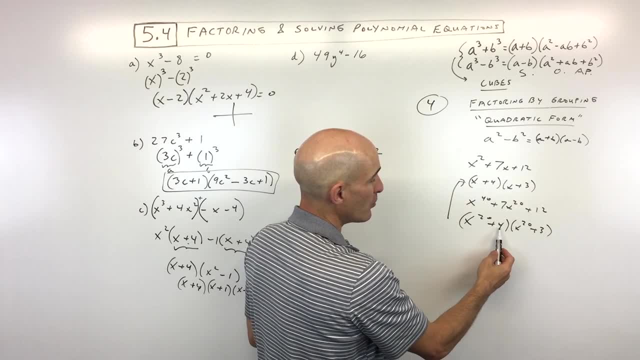 x plus 4x plus 3?? This is the same thing. It's x to the 20th, though, plus 4x to the 20th plus 3, because, remember, when you multiply you're adding those exponents. That's going to give you back the. 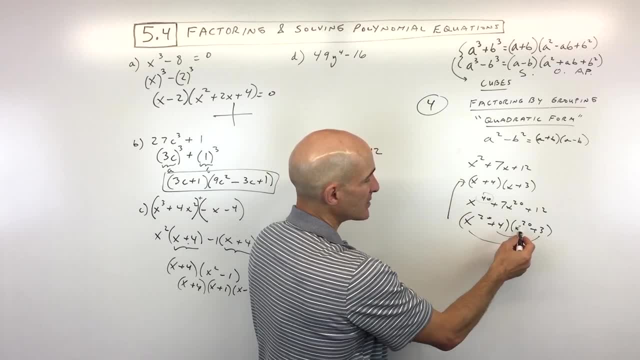 x to the 40th here. but when you do the inner and the outer, 4x to the 20th, 3x to the 20th, that's going to give you 7x to the 20th. So this is what they call quadratic form. It's just like 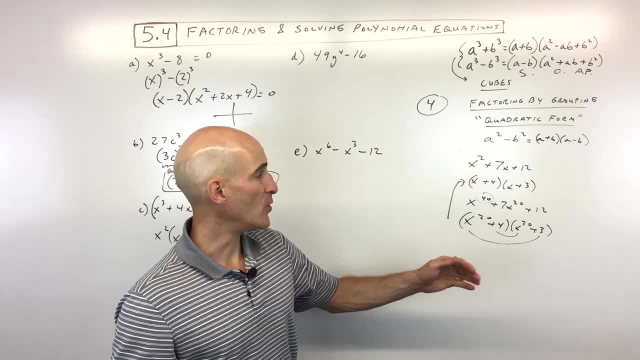 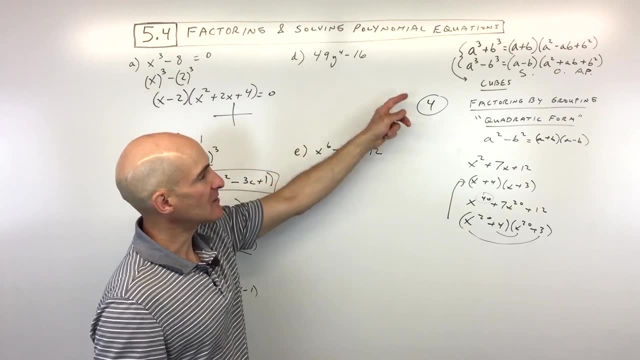 factoring a quadratic, a second degree polynomial, but we're just doing it when it's a higher degree. I'll show you some examples. So let's look at this. Let's look at letter d. When we look at this one here, it looks a lot like this formula here: 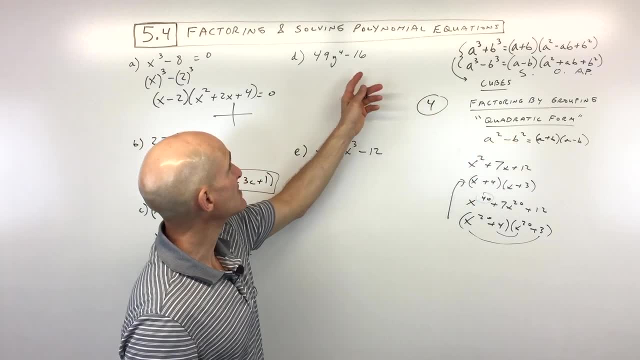 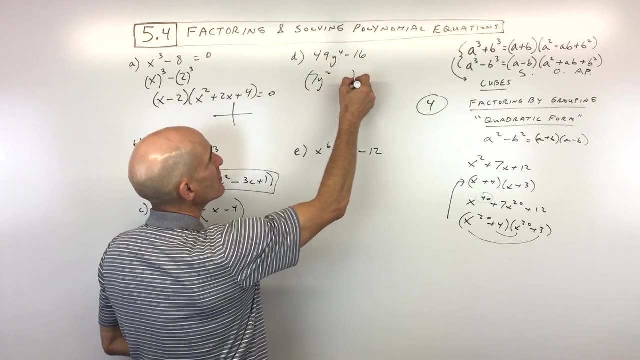 a squared minus b squared, the difference of two squares. The only difference is this is really not like y squared, It's y to the fourth, but if we take the square root of this quantity, we get 7y squared. If we take the square root of 16, we get 4, and we just make one of these adding and one. 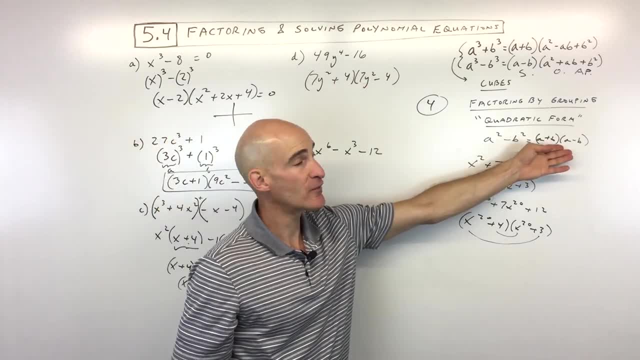 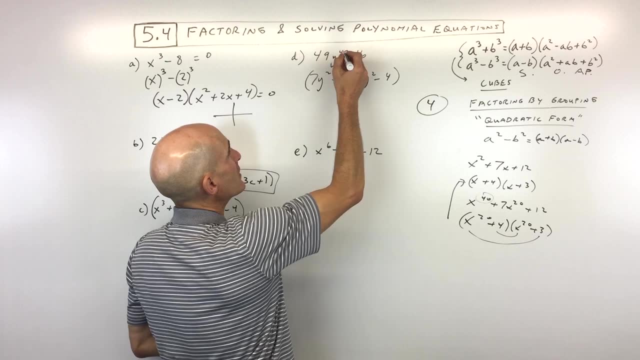 of these. subtracting, This is the difference of two squares formula, the sum and difference pattern. but all I did is see. even if I were to change this, so let's say, for example, the 40th, this would just be 7y to the 20th and 7y to the 20th. 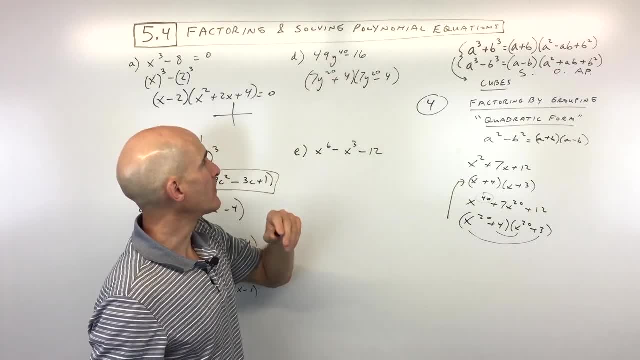 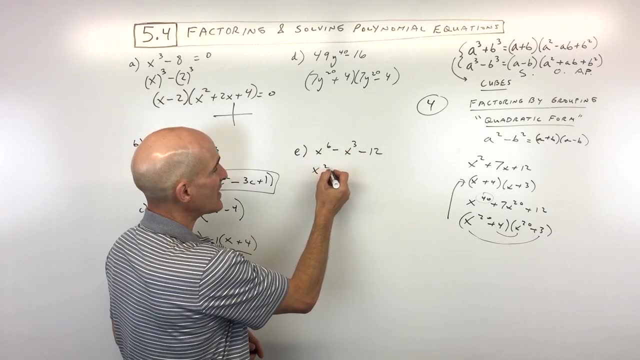 It's just going to be half of that exponent there. So let's look at letter e. Now this one x to the sixth minus x, cubed minus 12, would you know how to factor it if it was x squared minus x minus 12?? You know to kind of rewrite it like this when this: 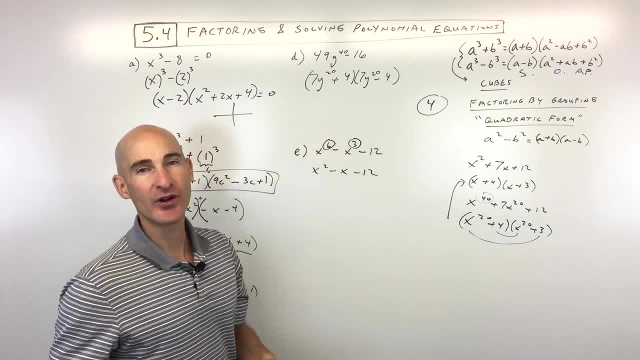 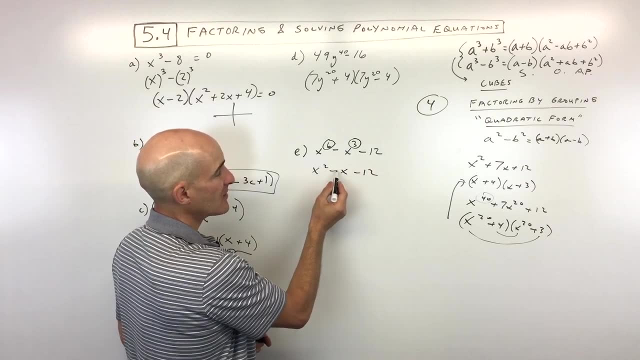 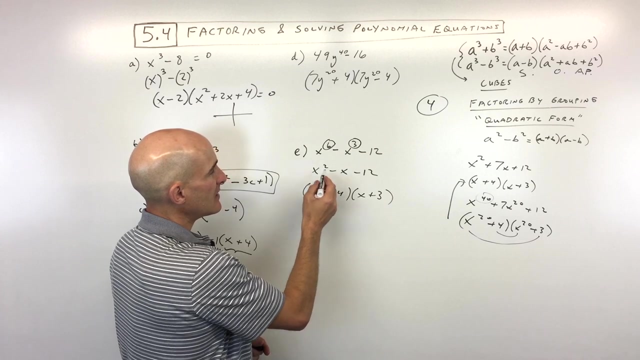 middle exponent is half of that leading exponent. Okay, so that's how you can recognize that quadratic form. What we're doing is we're saying what two numbers multiply to negative 12, but add to the middle coefficient negative 1? Well, that's going to be negative 4 and positive 3.. But in this case we 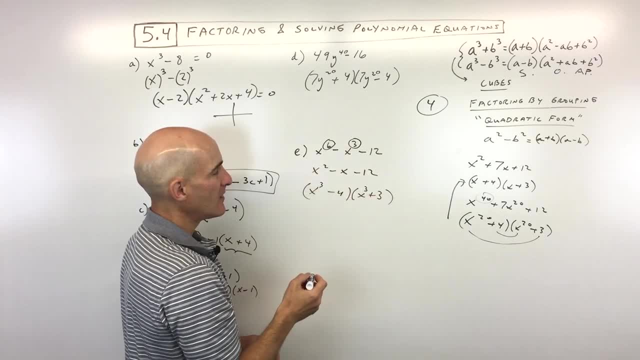 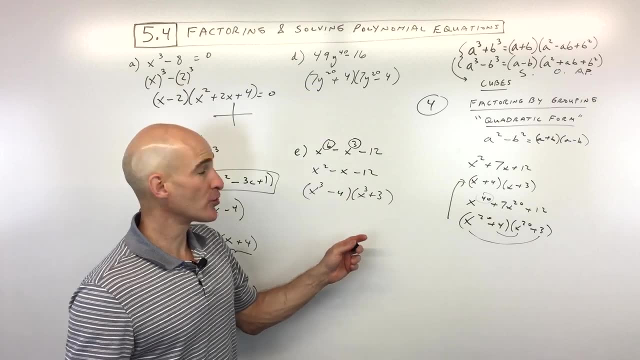 have x to the sixth and x cubed. This is going to be x cubed because when you multiply 3 plus 3 gives you x to the sixth. You add the exponents- We talked about the properties of exponents earlier in this course- And then, when you do the inner and the outer product negative, 4x cubed. 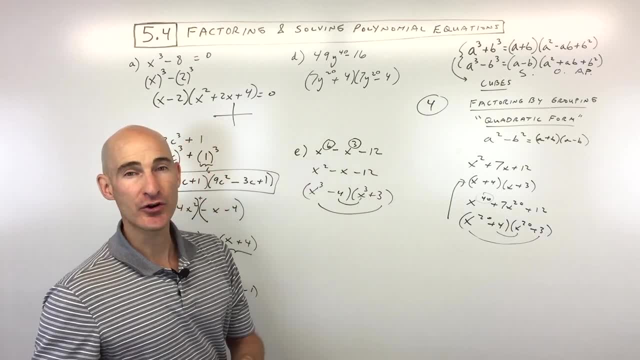 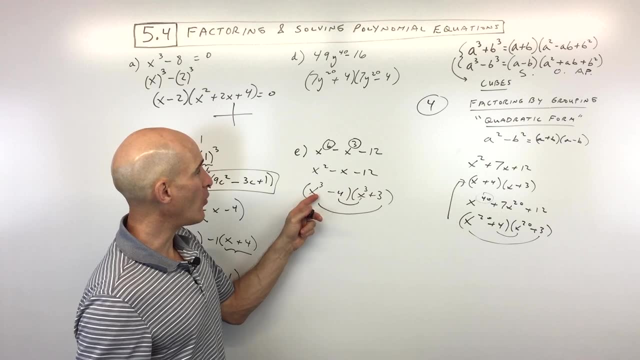 and positive 3x cubed, that gives us the negative 1x cubed, the middle term. So you can see, this is really just like factoring this second degree trinomial. It's just that now we've got it to a higher degree And again you recognize it by this middle exponent being half. 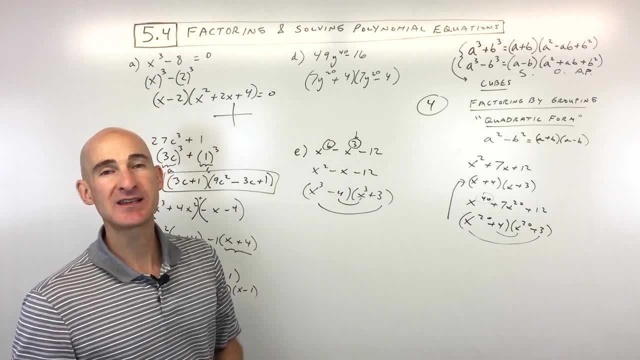 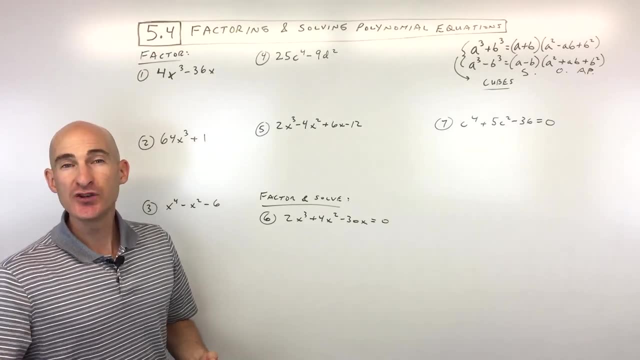 of that leading one, So let me erase the whiteboard. I'll put up some sample problems that you can practice on your own and we'll go over those so you can get some additional practice. Okay, see if you can pause the video and do these practice problems on your own to get some. 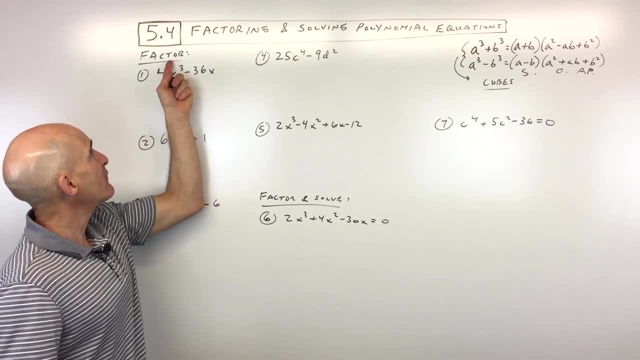 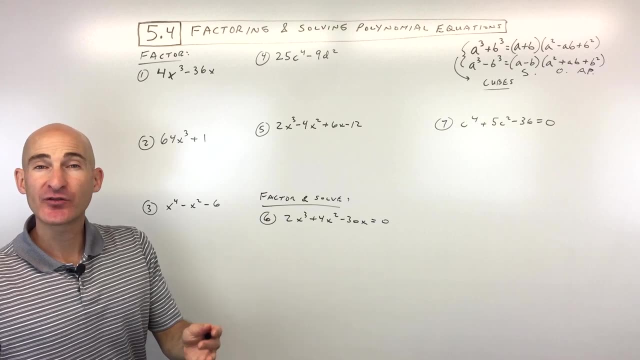 practice and experience. Number one: it says factor 4x cubed minus 36x. So how would you do that one? How would you factor it? Well, remember, the first step in factoring always is to look for that greatest common factor, that thing that you can divide. 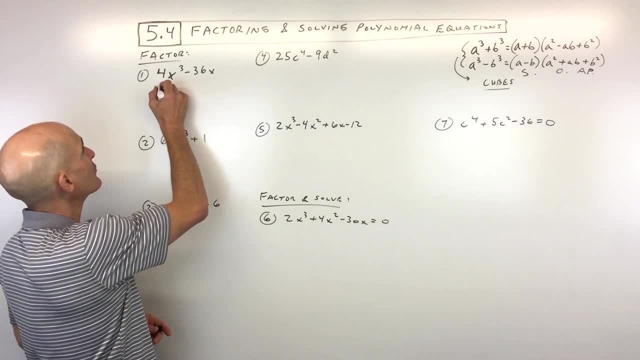 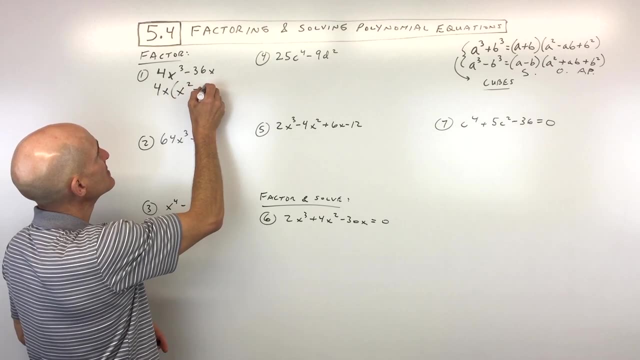 out of all the terms And this particular problem. it looks like we can factor out or divide out 4x, So we can divide these both by 4x. That's going to leave us with x squared minus 9.. Now 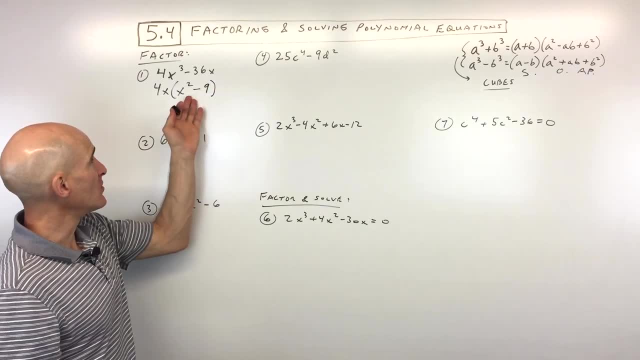 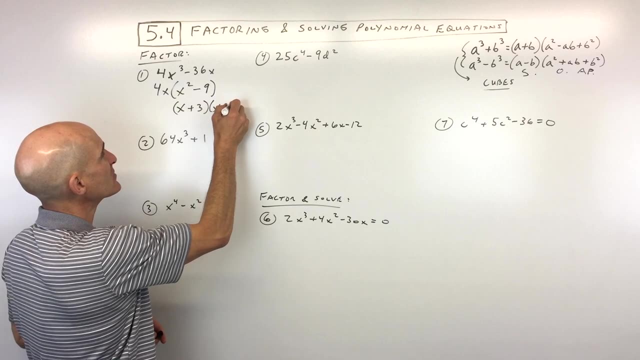 with factoring, you always want to see if you can factor further. So in this case we can see we have a difference of two squares, two perfect squares, which factors with the sum and difference plus 3x, minus 3.. I just took the square root of 9,, which is 3,, and the square root of x, squared. 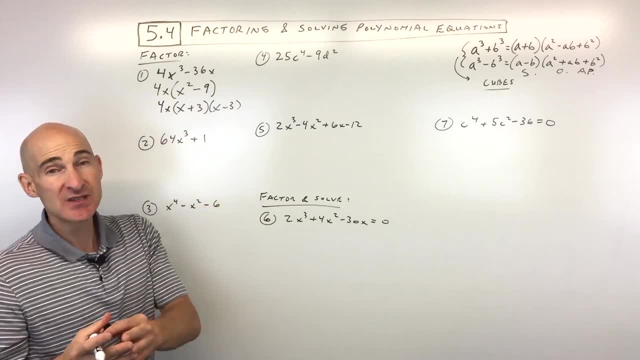 which is x, And we bring down that 4x. Now, if this was equal to 0,- right here, this quantity equal to 0,, then I would set 4x equal to 0, x plus 3 equal to 0, and x minus 3 equal to 0,. 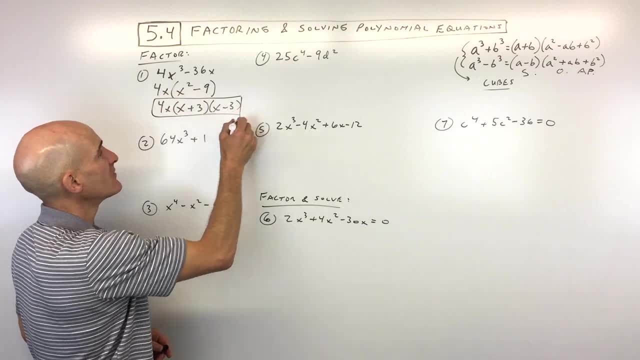 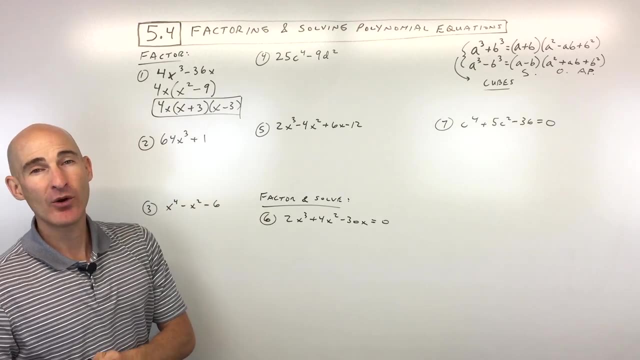 and I would solve, But for this one it just says factor, So we're just going to leave it like that. Okay, try number two: 64x cubed plus 1.. How would you factor that one, 64x cubed plus 1?? 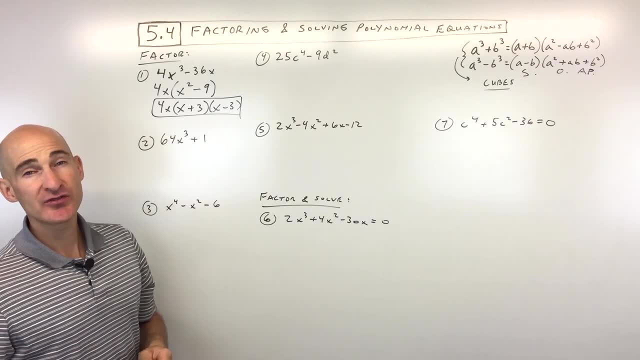 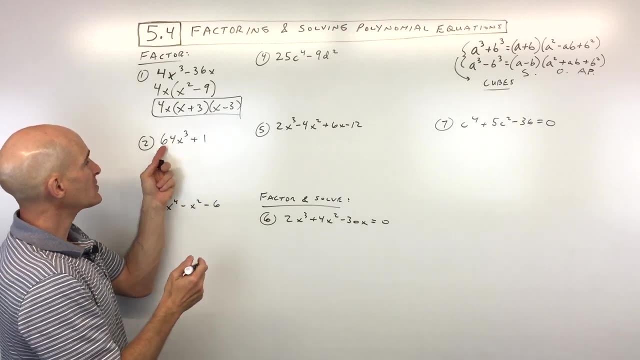 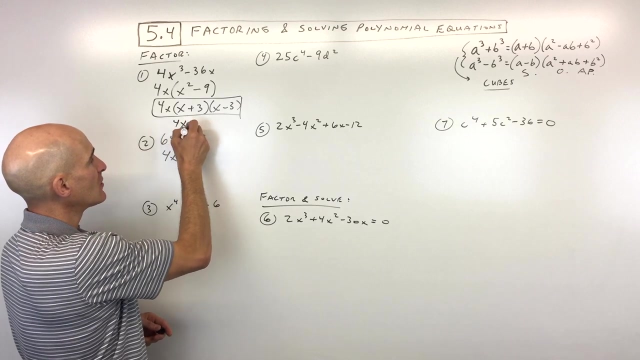 Well, first step is look for the greatest common factor. It doesn't look like there's a greatest common factor, but it looks like we have a sum of two perfect cubes, because the cube root of this quantity is actually going to be 4x times 4x times 4x and the cube root of 1. 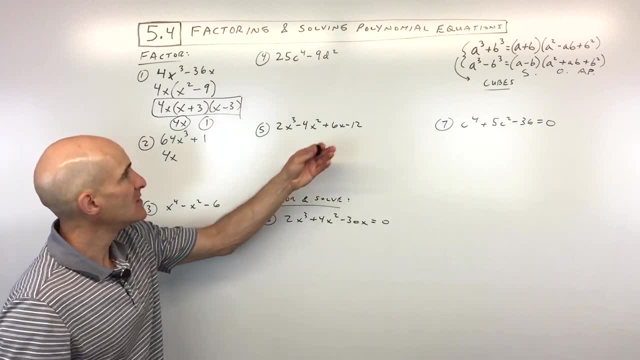 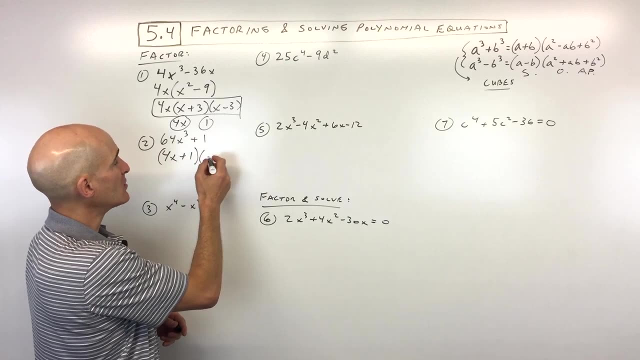 is just 1.. So this is our a value, This is our b value in this top formula here: the sum of two cubes. So I'm just going to expand this out: 4x plus 1, 4x squared is 16x squared. Okay, that's. 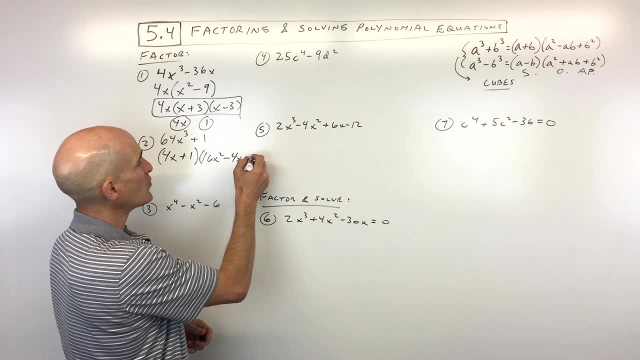 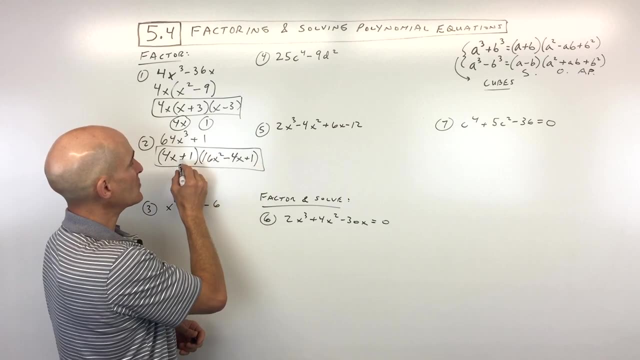 minus 4x times 1, which is 4x plus 1 squared, which is 1.. And so now we've got it factored, and I use that SOAP acronym: same opposite, always positive. So we're adding, so it's adding. 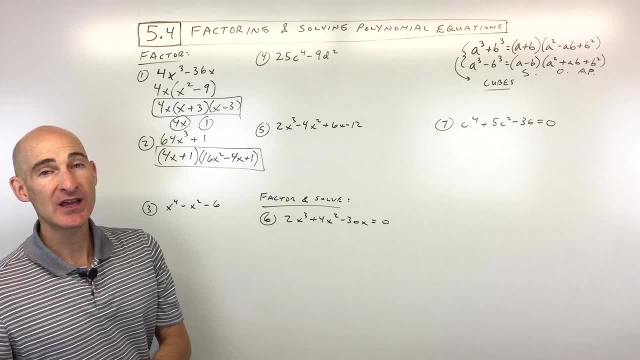 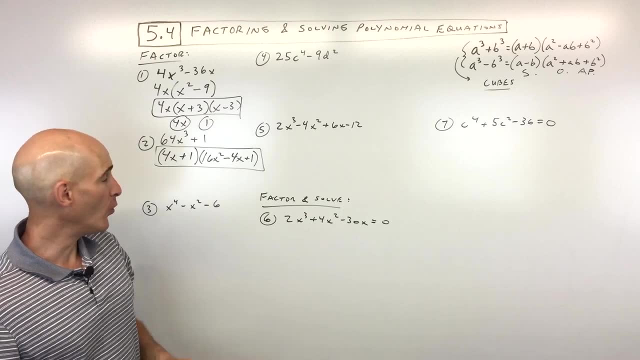 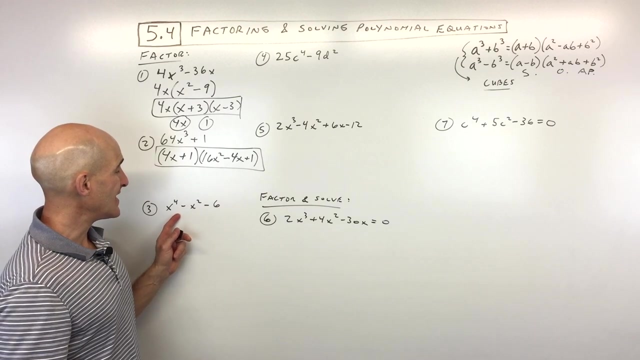 the opposite, subtracting always positive for the last one. Okay, so let's look at number three. So x to the fourth, minus x, squared minus 6, how would you factor that one? Well, you can see it's a trinomial. There's not a greatest common factor, but it looks like it's in the quadrature. 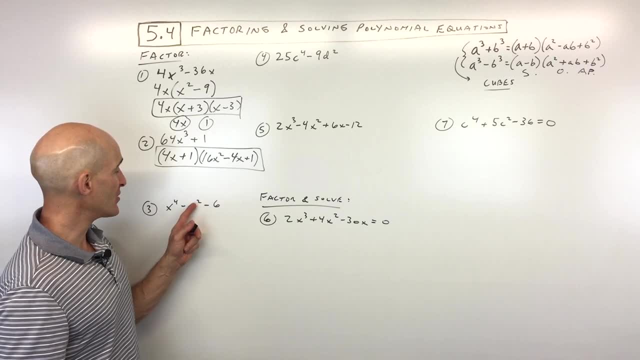 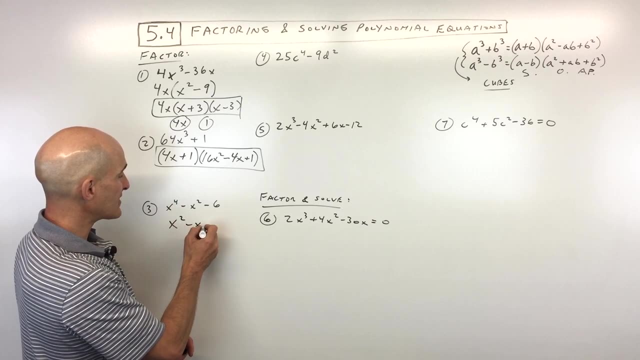 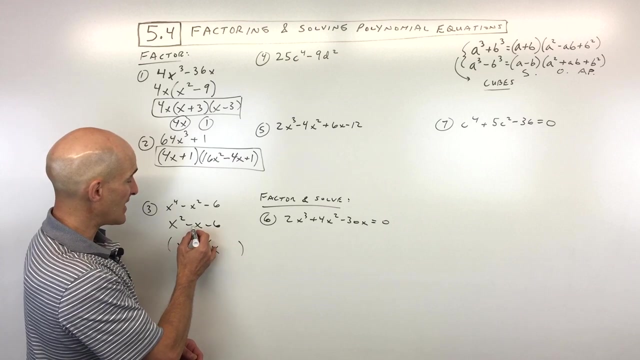 See how this exponent in the middle here is half of this leading terms exponent. So we're going to factor this just like we were going to factor x squared minus x minus 6. It's the same exact way. you'd factor it x times x is x squared What multiplies to negative 6 but adds to negative 1,. 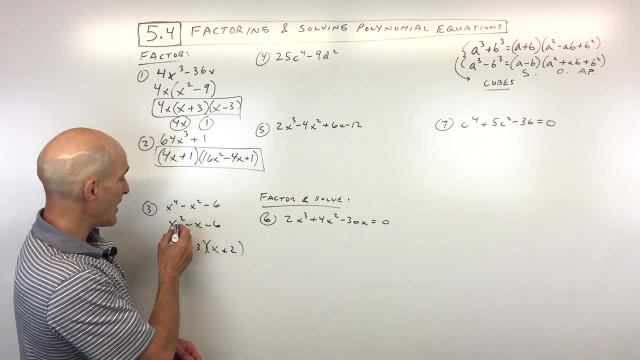 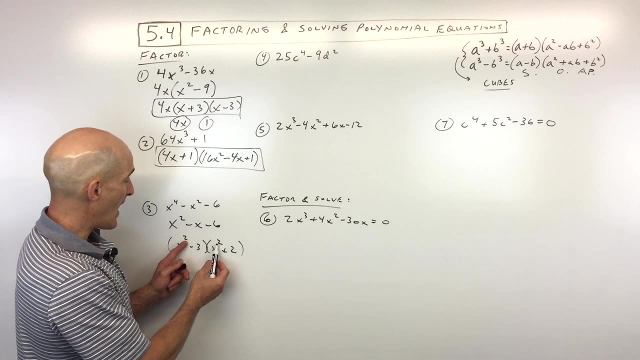 that's negative 3 and positive 2.. But because this is not x squared, it's x to the fourth, this is going to be x squared and x squared. Notice again: when you multiply, you add 2 plus 4.. And when we do the inner and the outer terms, that's going to give us back this middle term. 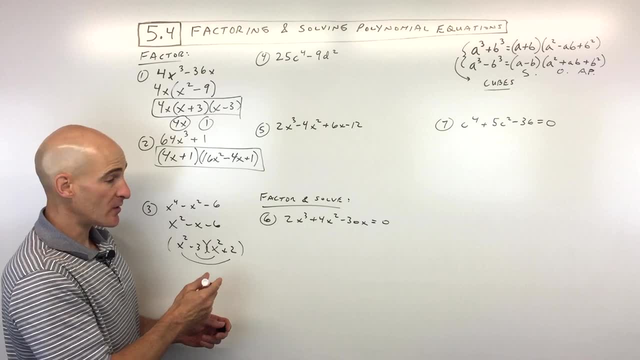 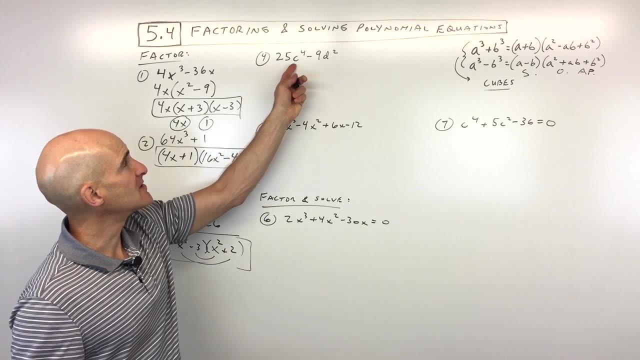 here. Now, if this was equal to 0, we would set each group equal to 0. But in this case it just says factor. So we've got it Okay. so let's go to number four. See if you can do this. one 25c to. 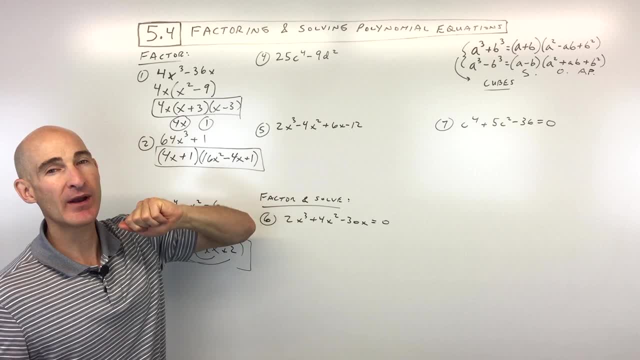 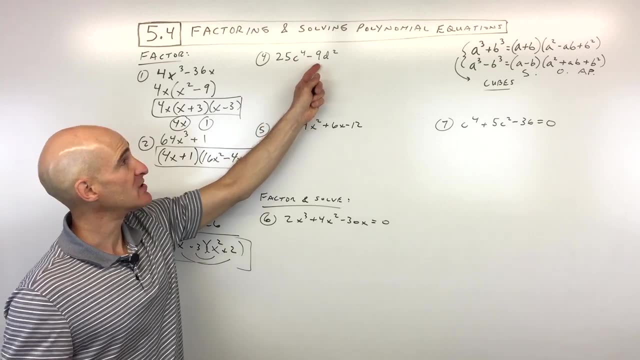 the fourth minus 9d squared. Okay, so what do you think for that one? How would you factor it? Well, there's not a greatest common factor. It looks like we have a binomial, two terms, and it looks like it's a difference of two perfect squares. So when we factor this, 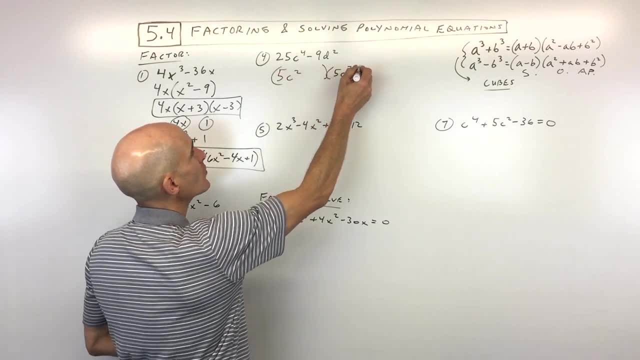 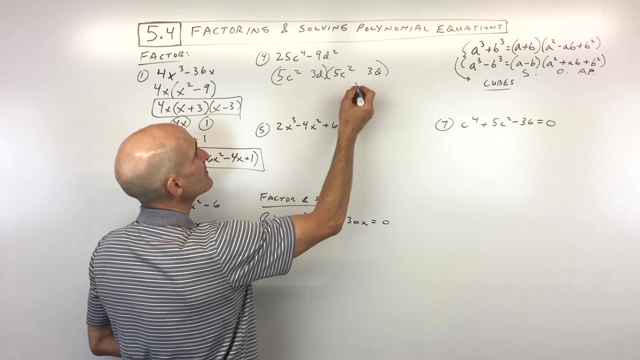 it's going to be 5c squared times 5c squared right, because these multiply to 25c. to the fourth, The square root of 9d squared is 3d times, itself 3d. One of these I'm going to make adding: 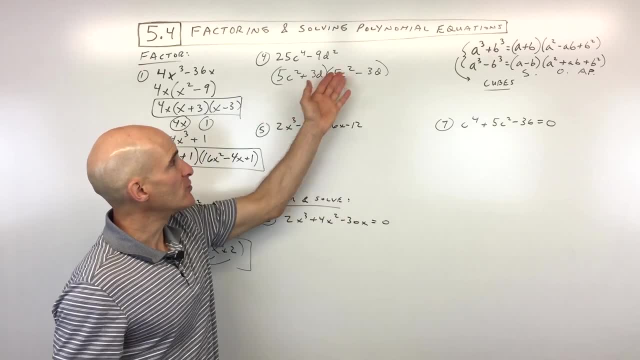 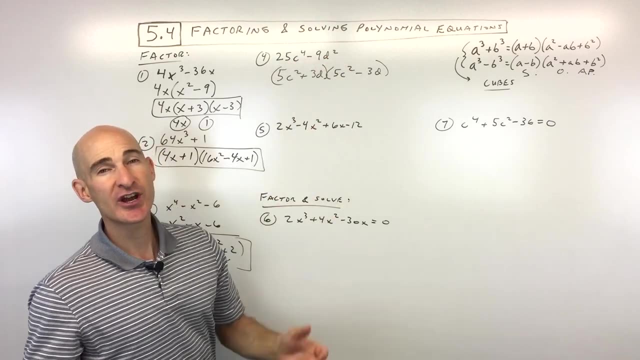 one subtracting. Now the nice thing about factoring: if you distribute twice here, or foil, or use your box method, any technique for multiplying out these two binomials- you're going to get back the original. So you can check your work right? So number five. 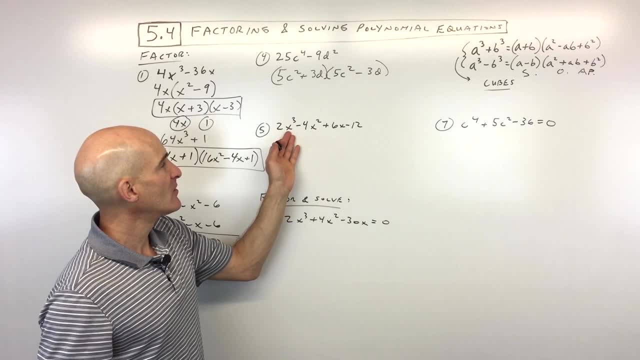 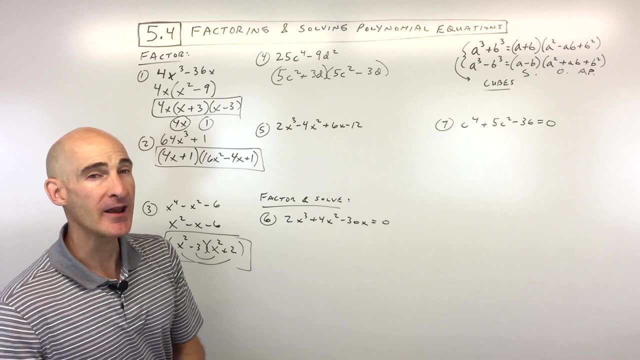 what do you think for this one? How would you factor this? So notice that we have four terms. That's interesting. So normally we have four terms. We think about factoring by grouping, but it looks like we could divide all these terms. 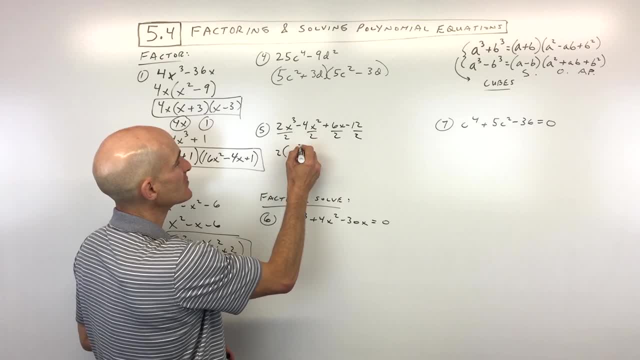 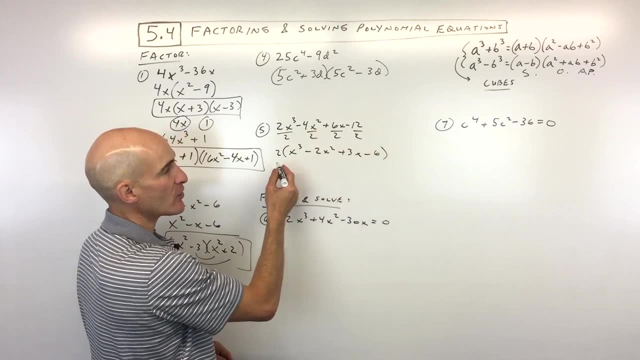 by two. So we're going to factor out a two. So that's going to leave us with x cubed minus 2x squared, plus 3x minus six. I just divided everything by two. I factored out that greatest common factor. But now what I'm going to do is I'm going to group the first two. 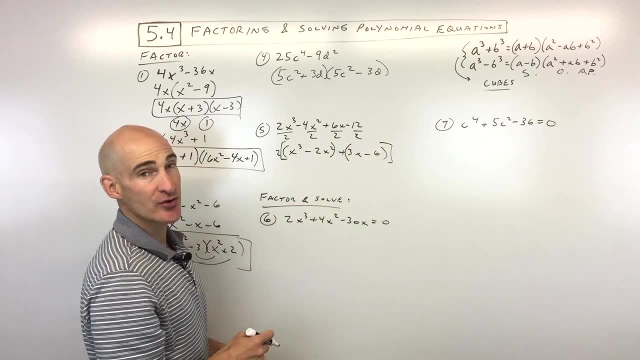 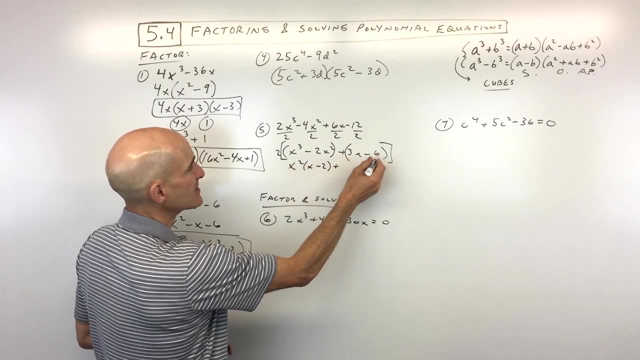 terms, and I'm going to group the last two terms. okay, I'm going to factor out the greatest common factor, which in this case is x squared, And in this case it's going to be three. right, We still have that two in front. We don't want. 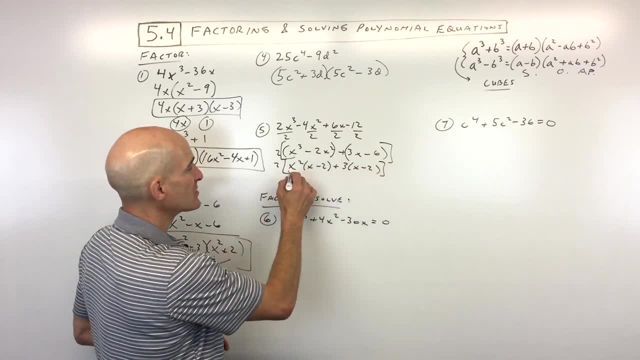 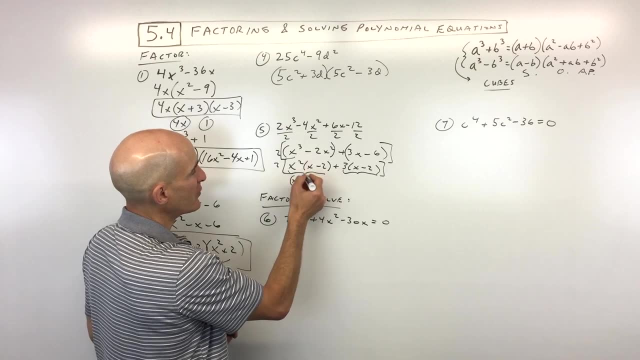 to forget about that. But notice how there's an x minus two in common in this group and in this group. So we're going to factor out that x minus two like a greatest common factor. where you can think about dividing this whole thing by x minus two, you'd be left with x squared If you divide. 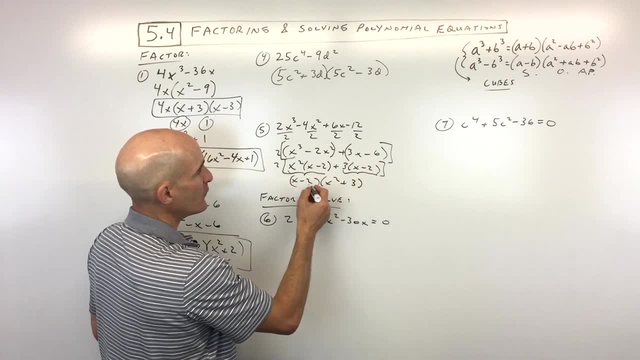 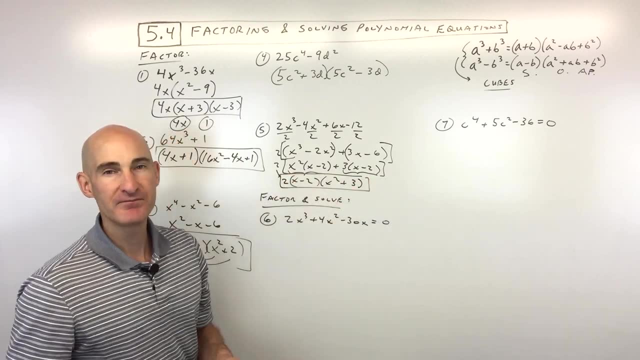 this whole group by x minus two, you'd be left with three. And again, if you foil this out, you're going to get back the original. But then we have to divide this whole thing by x minus two. just bring down that two, and now it's in the fully factored form. Okay, let's go to number. 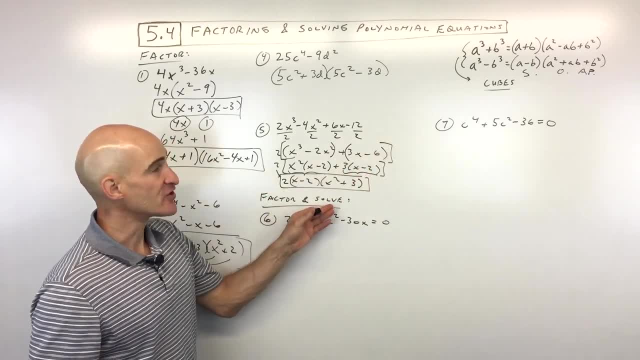 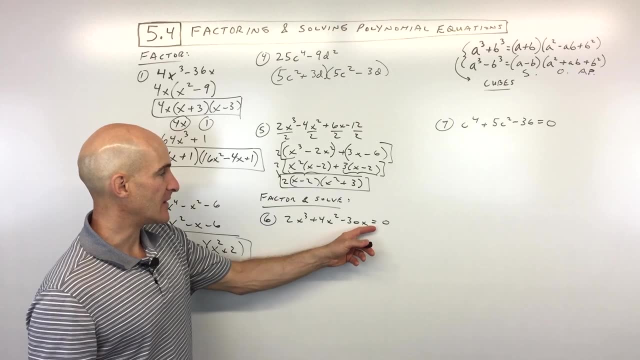 six and number seven. Here it says factor and solve. See how these are equal to zero. So that's kind of you know. when it's not equal to zero, usually it just says factor. You're not going to really be solving anything. But this is a trinomial and we want to find out what values of 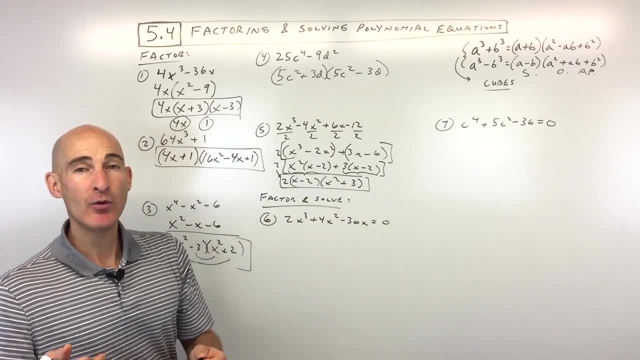 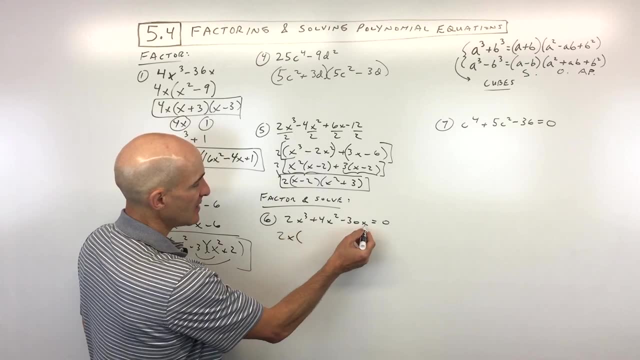 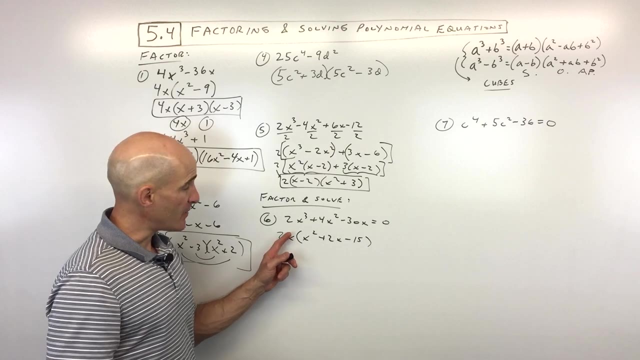 x are going to make this equal to zero. These are our x-intercepts when we graph our polynomial. So the first step with factor, remember, is the greatest common factor. So here I can factor out a 2x out of all these terms. Okay, now you can check your work by distributing that 2x to see if 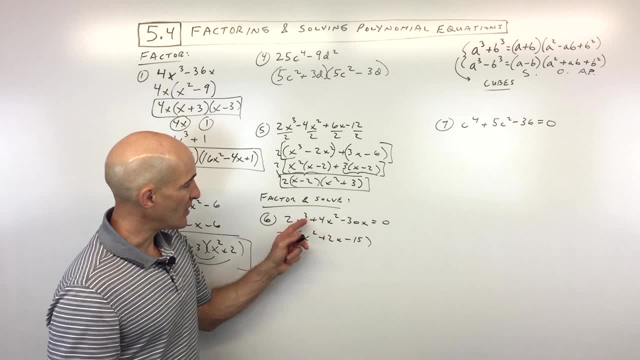 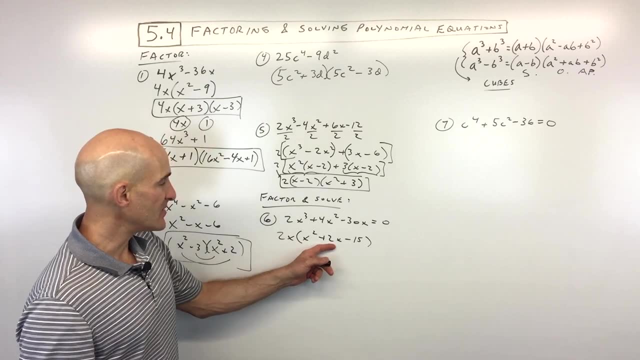 you've done it correctly, But you want to see. first look at the numbers. I can divide all these by two, and then I look at the variables. It looks like they all have at least one x in common. So that's how I factored out the 2x. Now the next step is: hmm, let's see what multiplies to negative. 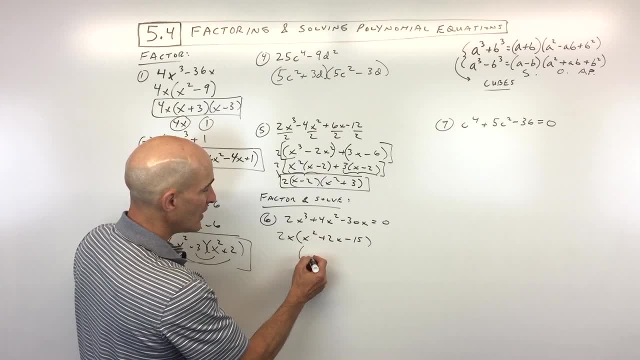 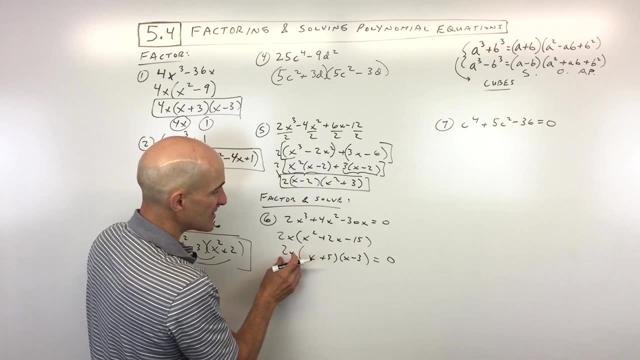 15, but adds to the middle coefficient two. That's going to be positive five and negative three. I'm going to bring down the 2x Now it's fully factored. but now what we want to do is we want to set each group. 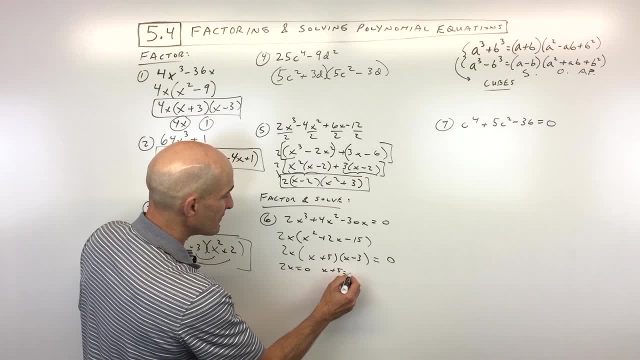 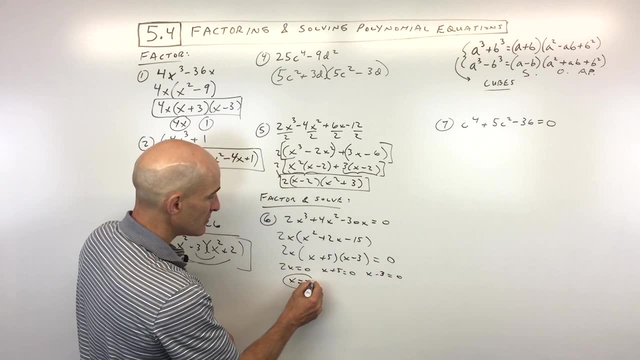 equal to zero. So we have: 2x equals zero, x plus five is equal to zero and x minus three is equal to zero. If I divide by two, x is equal to zero. If I subtract five, x is equal to negative five. 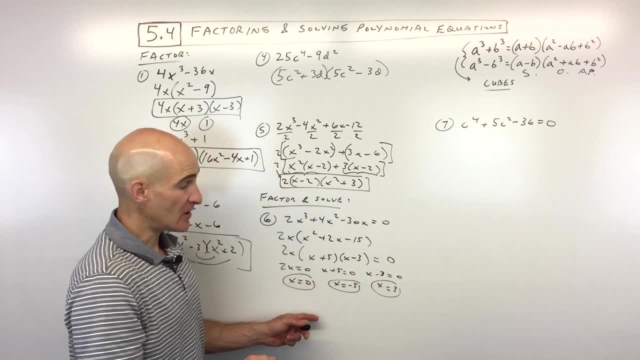 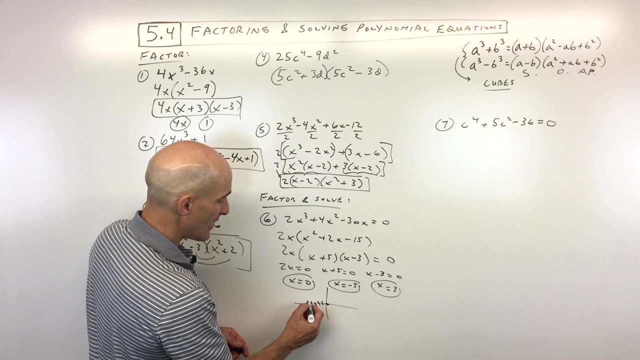 And if I add three, x is equal to positive three, And all this again represents is where the graph is going to be crossing the x-axis. It's going to be crossing here at zero, It's going to be crossing over here at negative five and it's going to be crossing over here at three. And 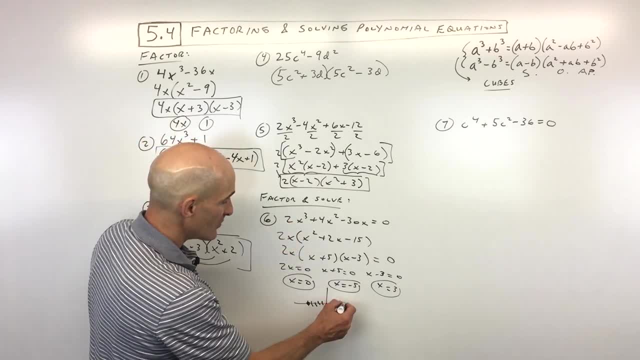 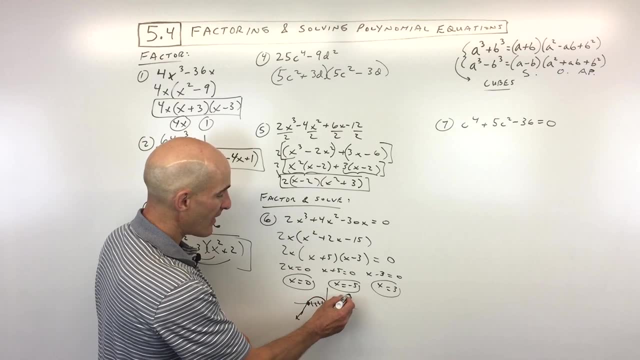 the leading coefficient is positive, so that means it's going to be going up to the right. It's an odd degree, which means it's going to go down to the left- the opposite direction- and it's going to look something like that. So we're getting a better idea about how to graph these polynomials. 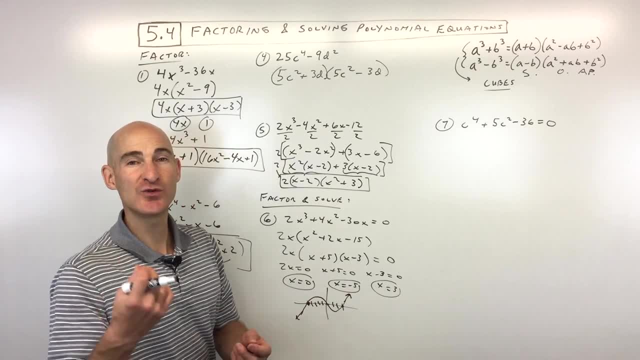 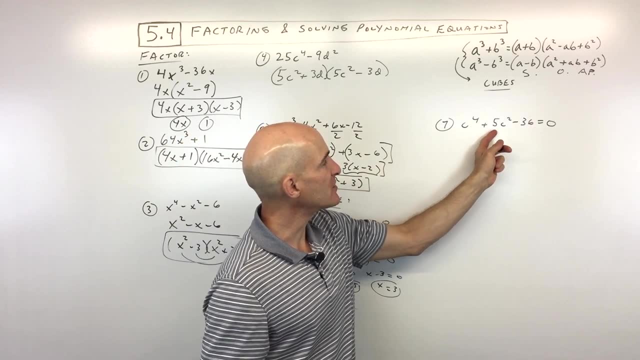 by finding the zeros and incorporating the n behavior which we learned in a previous lesson. Okay, last example for this lesson. See if you can factor this one c to the fourth plus five. c squared minus 36 equals zero. What do you think for that one? Well, there's not a greatest. 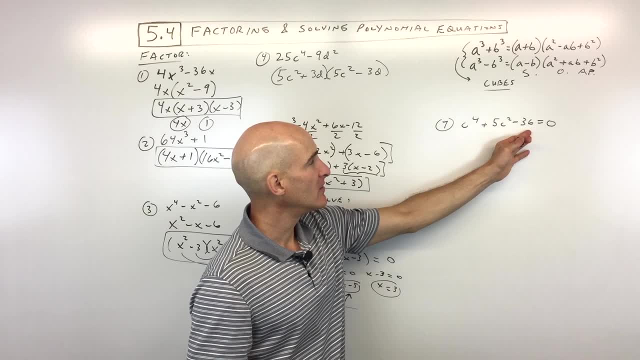 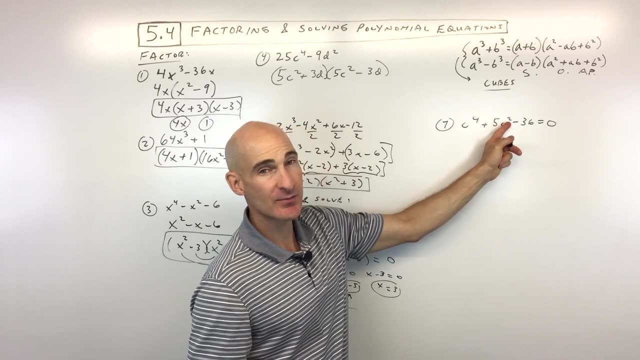 common factor. right, It is a trinomial, It's not a quadratic, though It's a higher degree. See, this is not c squared, It's c to the fourth. But we notice that that middle exponent is half of. 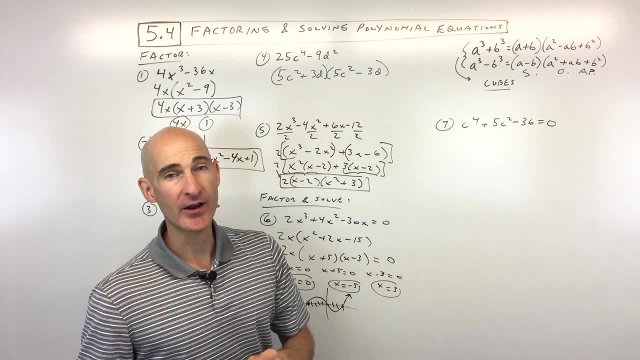 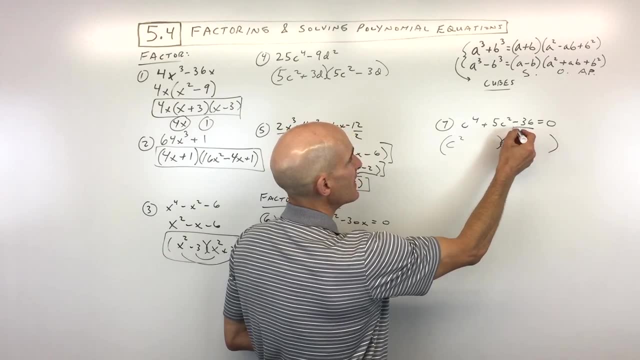 that leading exponent. So that tells us this is in the quadratic quote-unquote form, right? So when we factor this, it's going to be c squared times c squared. But what multiplies to negative 36 but adds to five, that's going to be positive nine and negative four. Now with factoring, 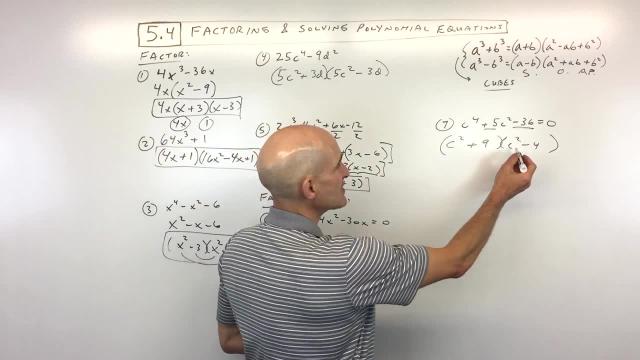 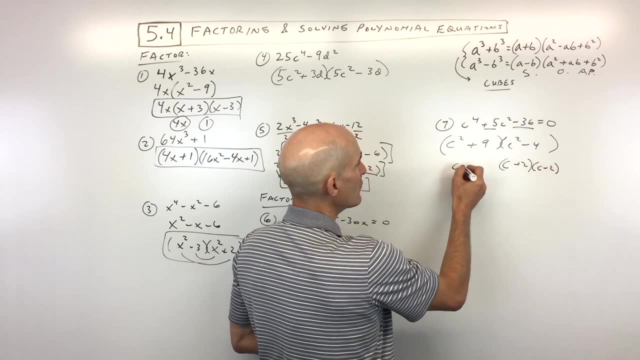 you always want to see if you can factor further. right, Keep going. We notice this is a difference of two squares. Okay, so this is going to factor to c plus two and c minus two. This one we really can't factor over the set of real numbers. 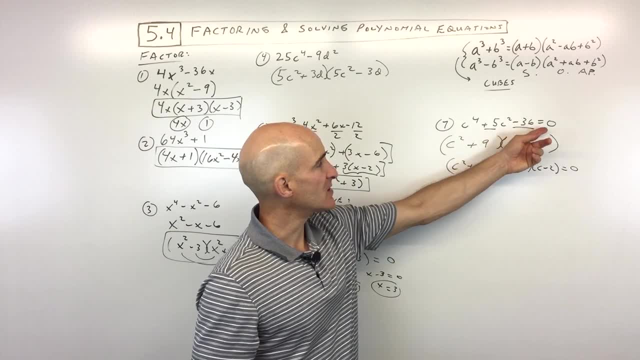 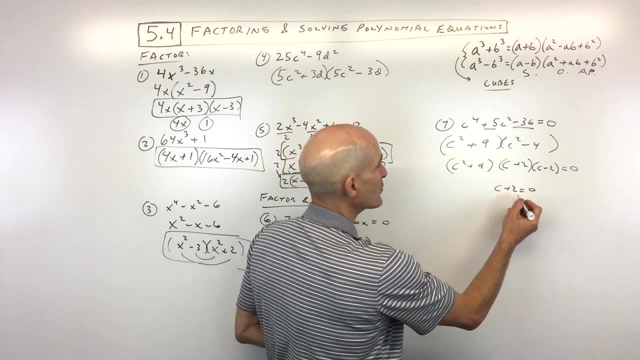 So now we've factored as much as we can, but we have to solve. So we're going to set each group, each factor, equal to zero. If we set c plus two equal to zero, that one's pretty easy. We just subtract two, we can see that c equals negative two. If we set c, 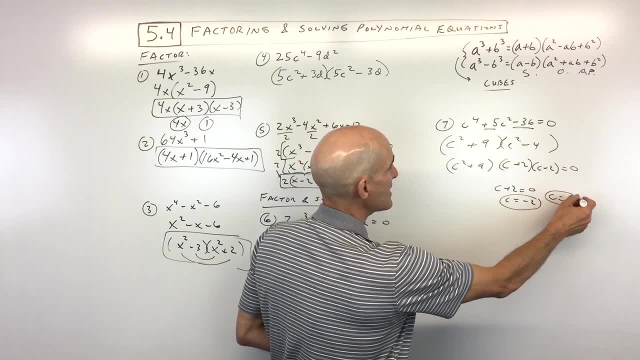 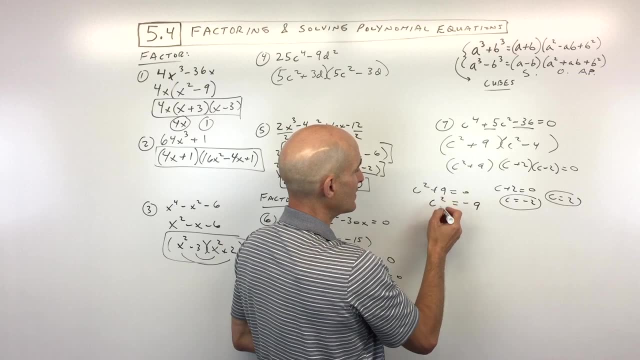 minus two equal to zero. if we add two to both sides, we can see that c is equal to positive two. But for this one, c squared plus nine equals zero. We subtract nine from both sides, It gives us negative nine. If we take the square root, we get two answers: positive or negative. 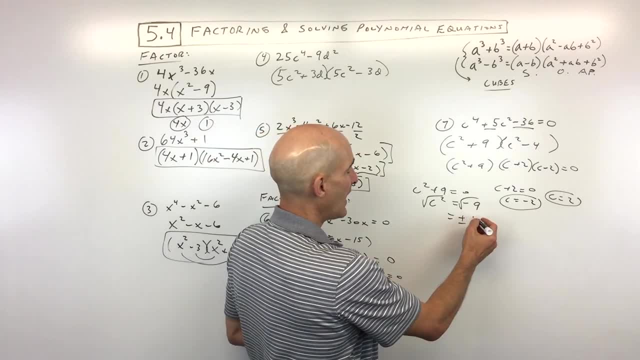 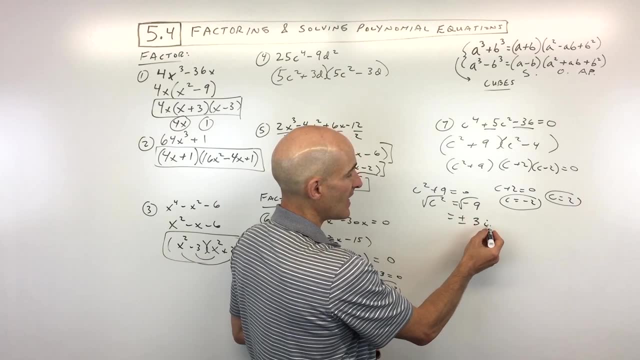 Remember, as soon as you take the square root of both sides, you get the two answers plus or minus, And the square root of negative nine is going to give you three. i, because square root of nine is three, but the square root of negative one is i, for imaginary right. So now we've got our. 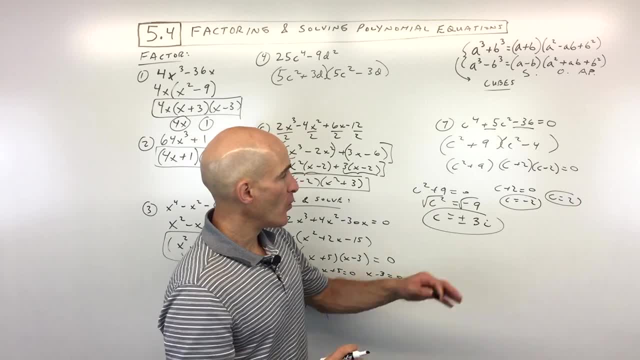 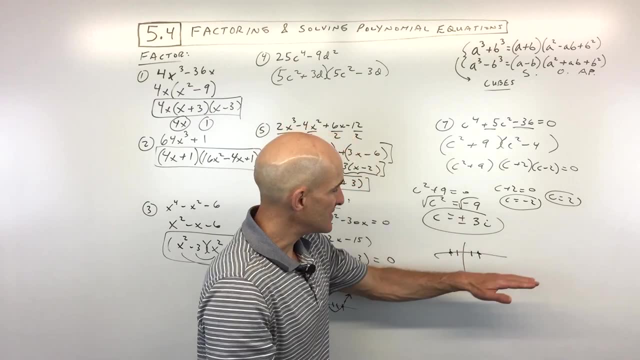 four solutions. The graph's going to cross over to the square root of negative one. So we're going to over here at negative two and positive two. but with the imaginary zeros it's not going to be crossing the x-axis at three i or negative three i. That's not going to be on our real axis here.